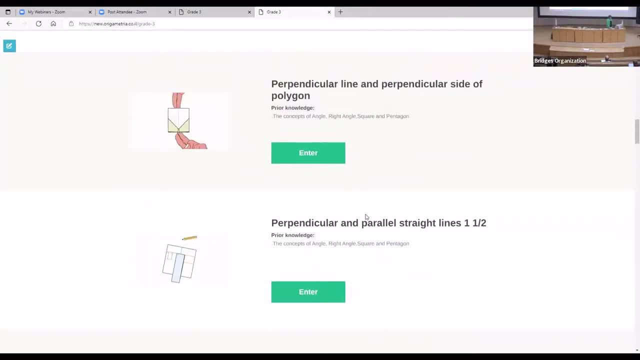 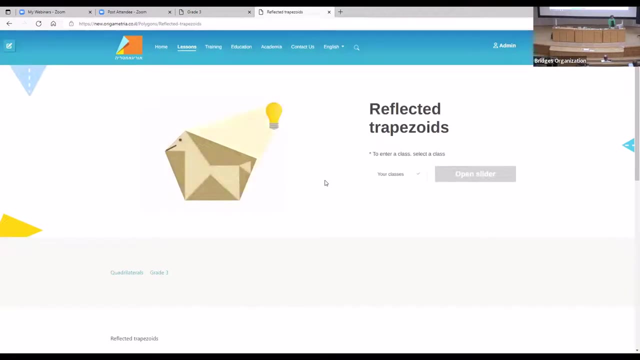 So, like the box, teach a perpendicular. So today I'm going to show you some lesson who call reflected propesium. You go to paper, you see the result. but when the teacher come to the class she opened the lesson, she choose the class, she prepare. It's called Helsinki Miri today. 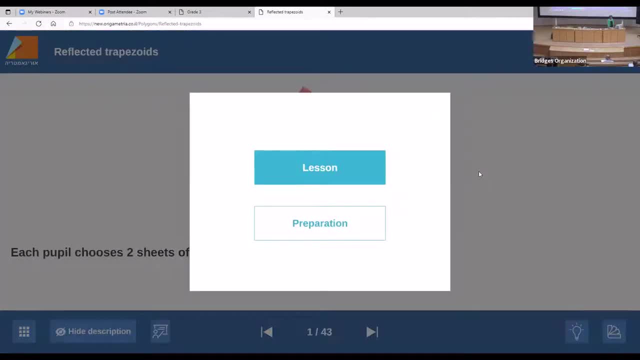 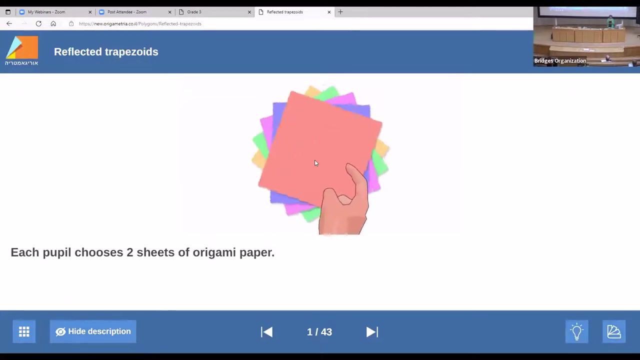 and she opened the lesson Now. usually she can prepare the lesson and write comment. Maybe she want to ask them some other question in the middle of a lesson. She can do it in the preparation. but because already prepared today, so I go straight to the lesson And now she's in house, she hands to the kids the origami. 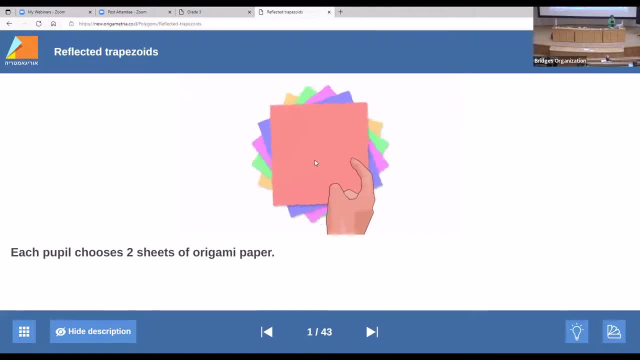 paper. So the children take the paper and she start to teach. You already got the paper. So one of the questions she asked them: what is the shape of this paper? So if I ask you, you say it's a square. And I ask you, why is it square? You always have. 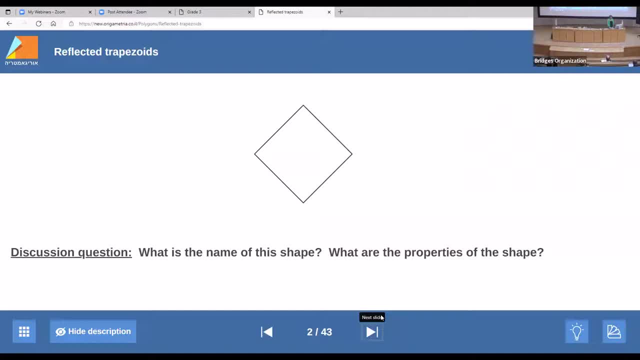 discussing question and answer and folding instruction. So you say to me: okay, it's a square, because all the side is equal, have a right angle, So it's a square. But how do you know all the side is equal? You say, okay, it's a square, because all the side is equal, have a right angle. 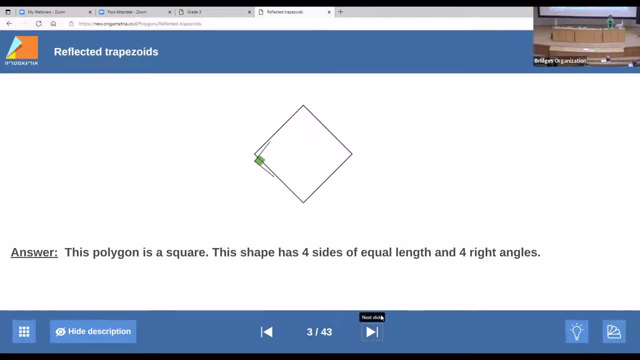 How do you know it's a right angle? We know from the PISA exam: many of the children fail because they say it's look like, Yeah, And we, with the origami paper I deal with this, look like the children work with the hand and the virtual world in the same time. So how we can do it. 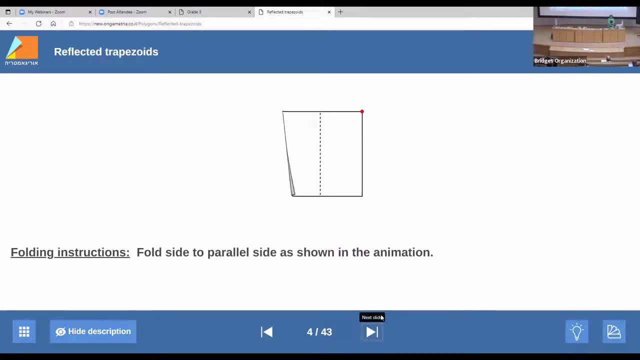 how we can know this is equal side and right. So what we do is that we we'll take the small page that's better at that side, Then we sew it with the long side of the paper that you buy, So it's more regimented, and we have a point in the middle of the Parkett side. the back side is equal to the top and the bottom side is the only left. We are guessing right. Hold on, We are guessing right. So now that we've seen all the other forms here, we can folded. now for practice. So I ask you to take one of the paper you have and fold one side, extend to the parallel side. 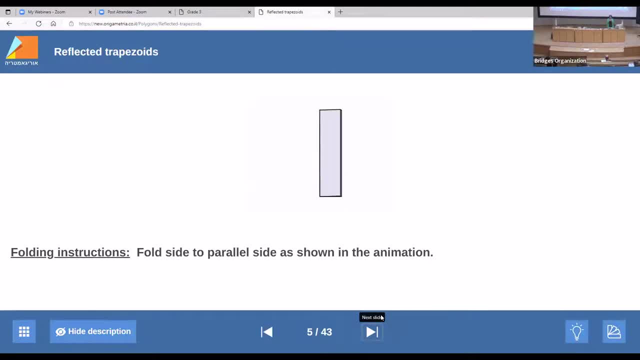 the parallel side And then, after you did that, you put a sign of a right angle only on one corner. So if you see the- we call it- paper measuring tool, And every student have it in his bag. If he lost it it's easy to make a new one. 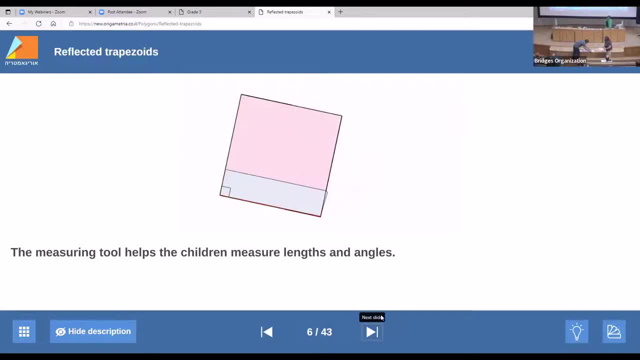 So now he can check that and say, yes, all side is equal and the angle is a right angle. So after he took the sign of a right angle only on one corner, he put a sign of a right angle only on one corner. So after he took the sign of a right angle only on one corner, he put a sign of a right angle only on one corner. So after he took the sign of a right angle only on one corner, he put a sign of a right angle only on one corner. 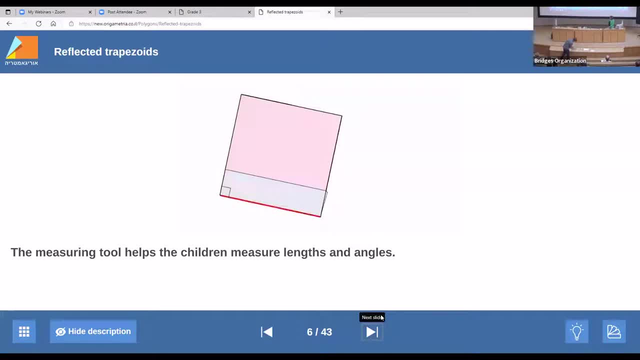 Then we know that. he knows it: Everybody have a square, Somebody don't have a square. Okay, So the measuring tool. this is how we start Now. the children don't know what we fold. You see it in the beginning, when I got into the lesson. 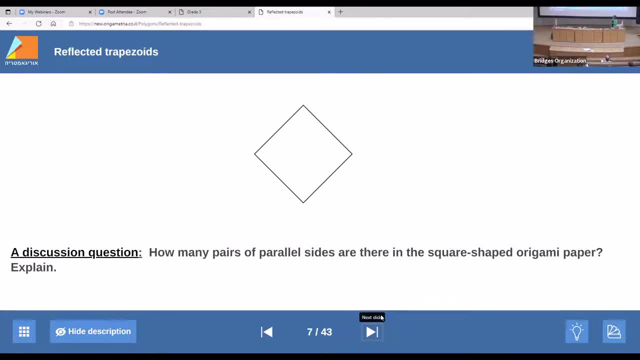 Why they don't see it When the teacher get into the lesson. the name of the lesson is reflective trapezium. It doesn't say what's the model We fold. If we want the children's imagination to work- and we know the children have high imagination, they have more cognitive ability and it's important to develop the imagination. 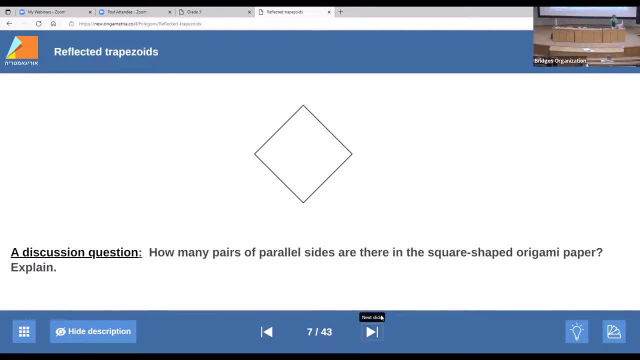 So we don't tell them: oh, we fold now a horse, Now we fold a bird. We don't tell them what we fold. What we fold today, It's a prize. So each time the paper changes they get a different model. 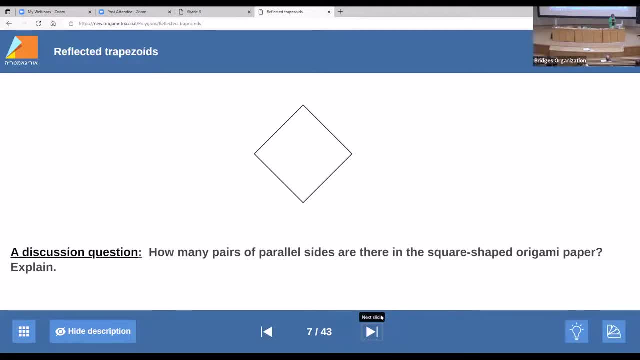 So now I ask you how many pairs of parallel sides you have in your paper and how you check that. So you tell me, yes, there is two parallel sides, two pairs of parallel sides. This is one of them, and this is another one of them. 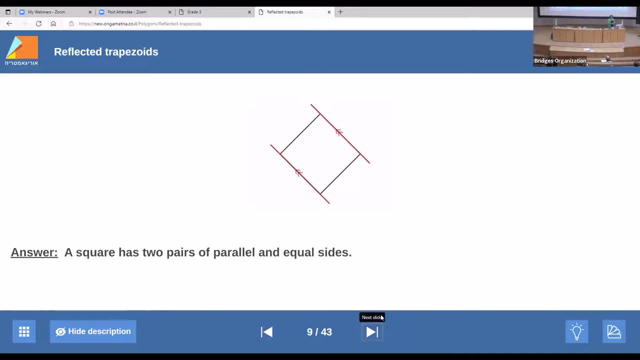 But how do you check they are parallel? Why? Why, If you show them in the square, all the children say it's parallel. Show them a rhombus, say it's not a rhombus. a parallel. yeah, It doesn't look like. 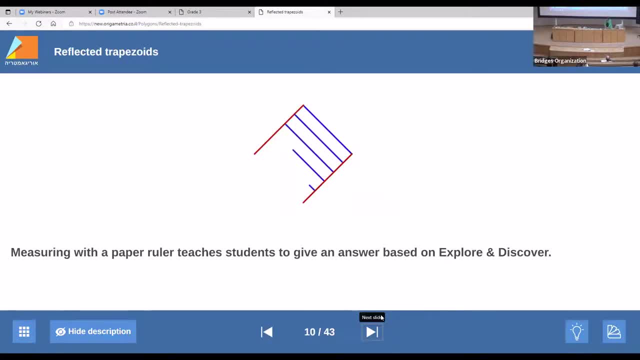 So we teach them to take the measuring tool and make a particular line between the two sides, and then you know the distance between the two parallel sides is equal. So now we fold. Take the other paper you have and fold one vertex to the opposite vertex. 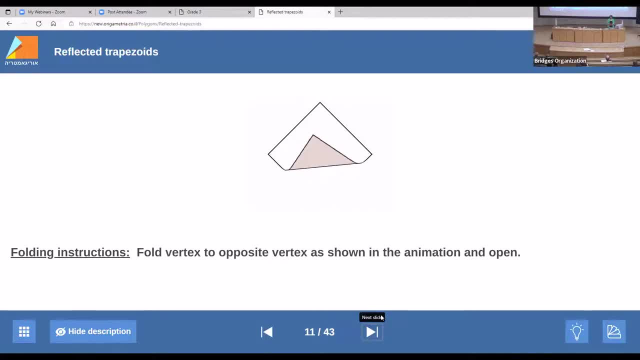 Now, I don't speak origami language Because while you come to teach, you want to teach them with a mathematics language. One of the beautiful comments I heard from teacher: they feel like they and the children have speaking the same language, because the children can read that. 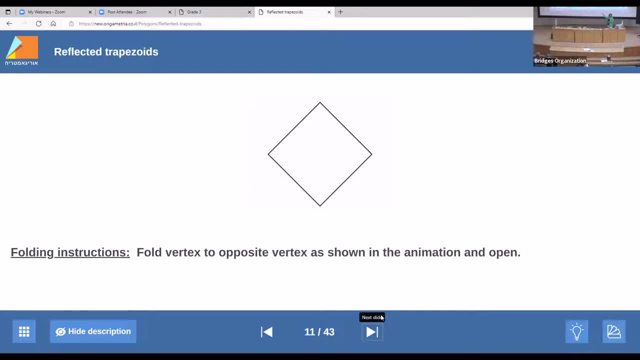 They read the question, They read the instruction, They read the answer, And this is very important because many times we need to give them a good mathematics language and they get used to that. So now we fold it and open it. And now what we do? we fold the side to the symmetric line. 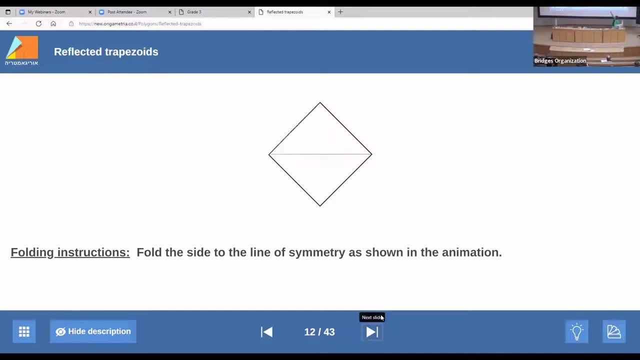 Now, when you fold it, make sure you fold in the same direction. you have here Now, if you see the light, the balls, how we call it. if I put the mouse here, it's a comment we give the teacher in the lesson if she want to remember something more. 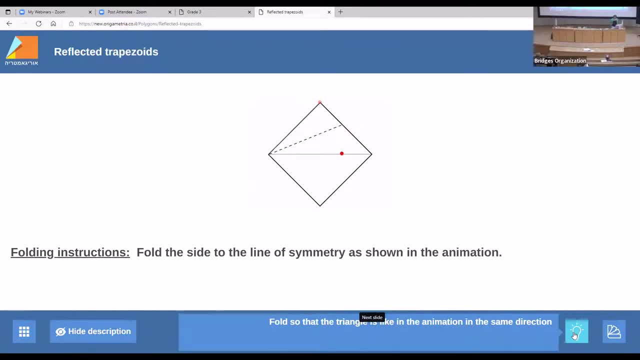 So now I tell the teacher: make sure the student fold it in the right direction. If I move the mouse it disappears. Okay, If the teacher put her mark she will see it in the other side. So after you fold it, I asked them how many pair of parallel side you see in the shape here. 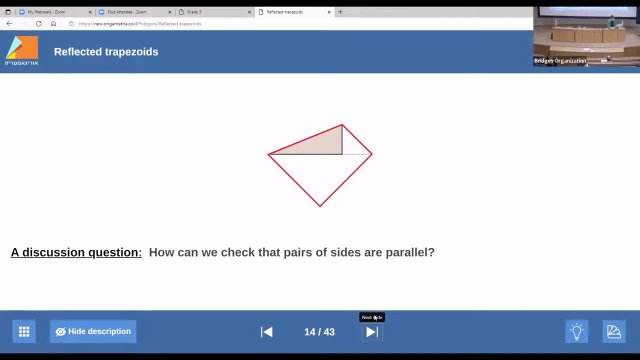 So the children checked it. How you check that? How you check it In the ruler? Yeah, Paper rulers. So what we do? we put the paper rulers on the shape we did and we mark it And we see the two sides are parallel to each other. 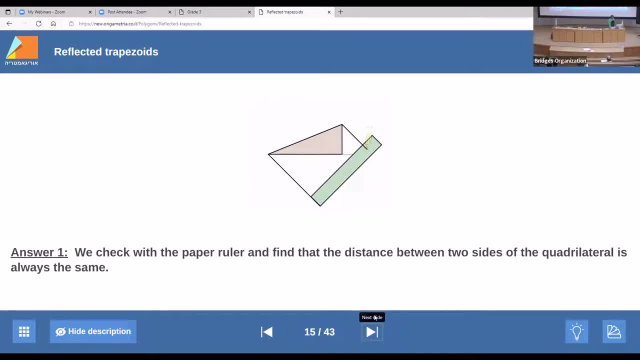 If you check it, we know it. So now we check the other side. No, this sorry, This is the parallel side. This is how we mark it. And now we check the other side. Okay, And now we see that if we continue, the two lines can meet. 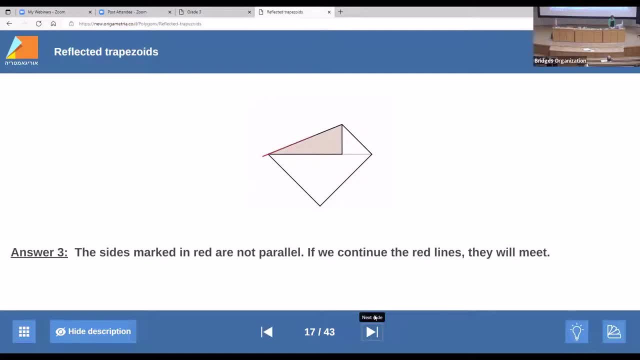 So this is not a parallel. So just now we say: what is trapezium? Part of the? I remember I teach in Los Angeles and ask the children to make a square and ask them what's that? They say it's a square. 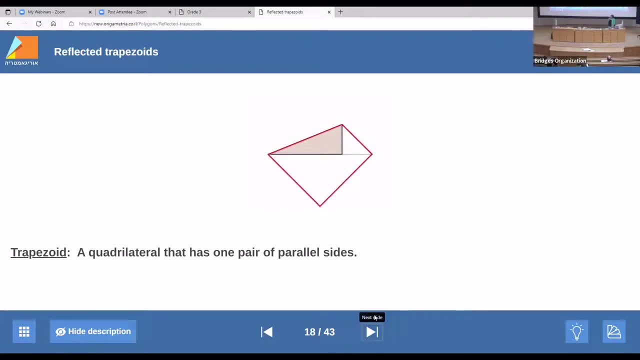 And ask them why it's a square, And they say: because the square. they try to remember what the teacher told them. If you teach by repeating by memories, you teach nothing, But if the student investigated and checked it, they never forget it. 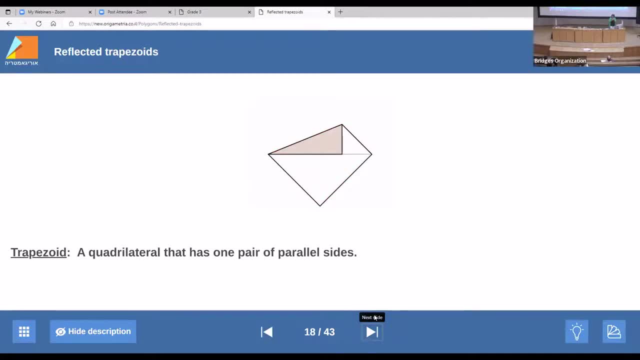 So here we check the parallel: how many pair? and we saw in the square they have two, and we saw in the trapezium we have one. So this is a parallel. So this is how I build the knowledge. 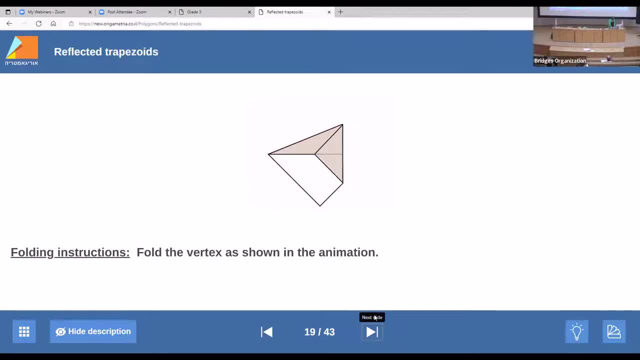 So now what you need you to do to fold the vertex is it show in animation. Now I want to show you something more about this animation. He worked very hard on it. The animation will repeat again and again, and again and again. So if the teacher want to go between the children, 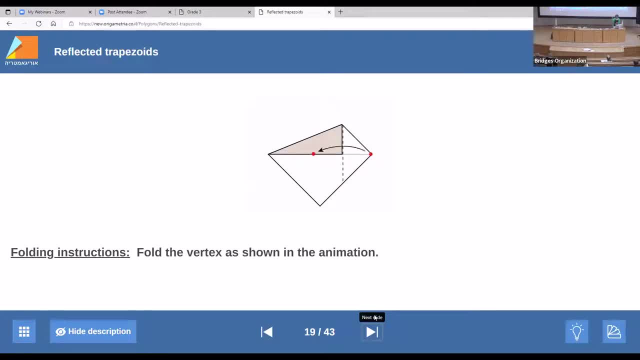 and see that everybody is okay. She can the animation continue to show it again and again so the children know how to do it. The model is created by Paul Jackson and he do all the work with the animator. Okay, so now how many pairs of parallel side? 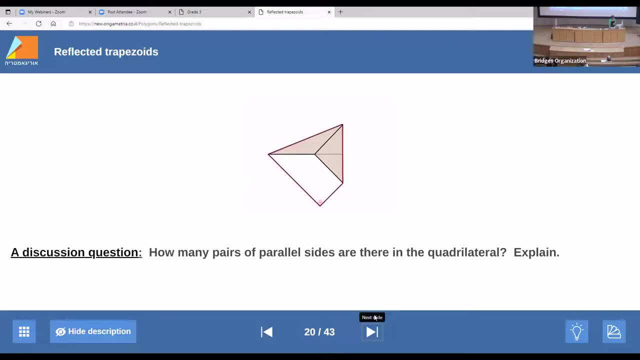 we have in this shape. So how we check that? So again, we look at the two sides and we see that if we continue they can meet, And if I see the other side they also can meet. Now it's look a bit like trapezium, yeah. 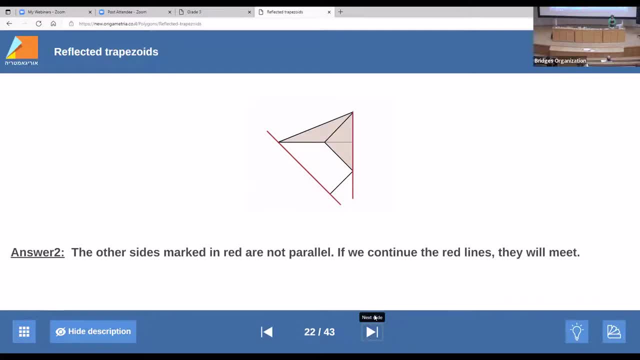 If you ask children, they say trapezium, but it's not because it doesn't have any. So when the children check that, they never do mistake. So it's quadrilateral but it's not trapezium. So now we fold another vertex. 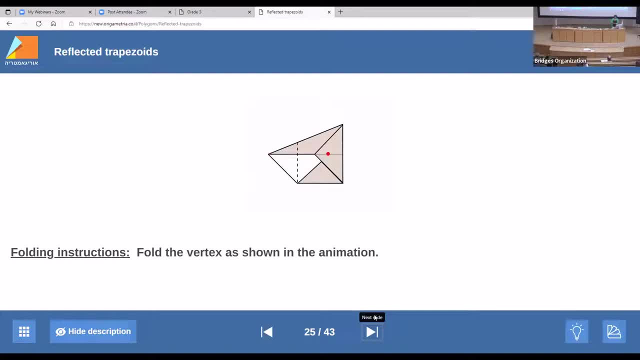 Now, when you fold the last one, you need to make sure that it's be exactly line up as you see in animation. Now, if I ask you, is it important to accurate in origami? Probably all of you will say yes, it's very important. 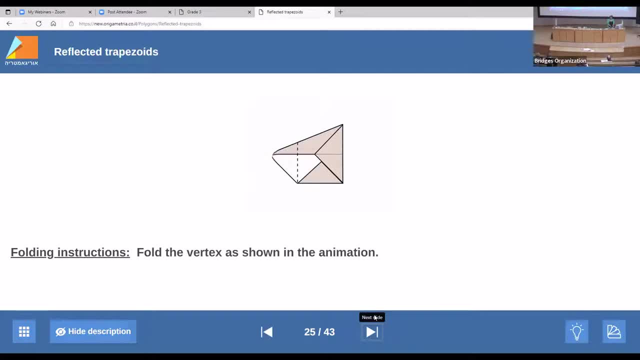 And I say to you: no, why not? People who get annoyed from if they are not folding, accurate? it's people who very, very accurate. They want everything to be precise. People who don't accurate: they just fold and say it's okay. 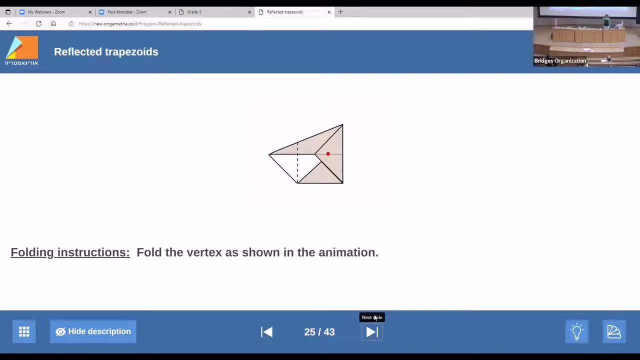 They don't see it. If I come and make a comment to them, they get frustration. I never saw anybody who learned from frustration. That's why I never check. And the student asked me: is it accurate? And I say I don't know. what do you think? 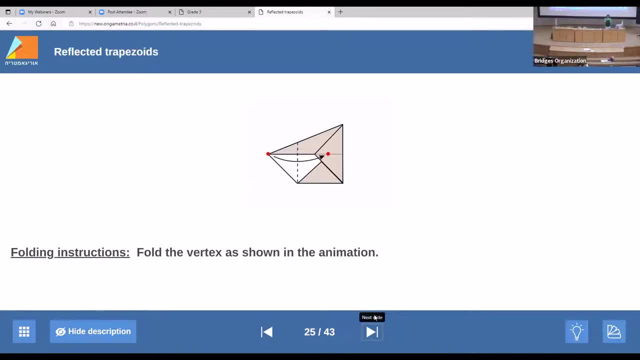 Is it accurate for you? Is it okay? No, it's not okay, so fix it. It's not me, it's you, it's your work. Another thing we do: there is a lot of method that I don't have time. 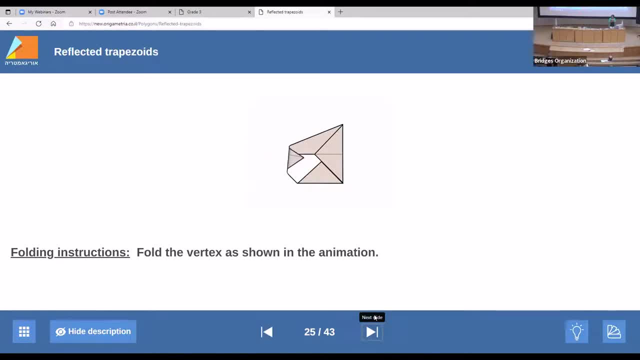 to tell you about it because origami come with an important method so it can make the student feel good about their work. We never touch the children work. I don't know if somebody come and teach you origami and they couldn't make it. 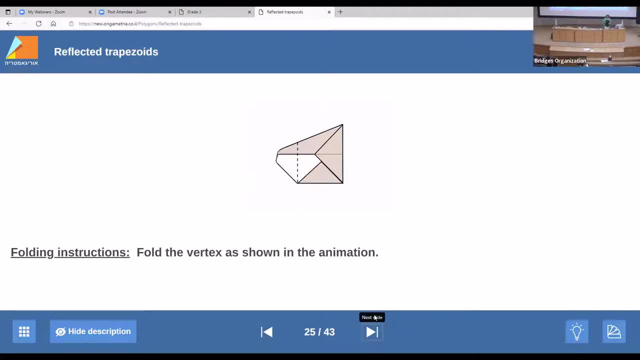 then they took your paper and make it. it's terrible. When I trained teacher, math teacher, and I really all the time tell them you're not allowed to teach, to touch the student work. So they tell me they put the hand behind the back. 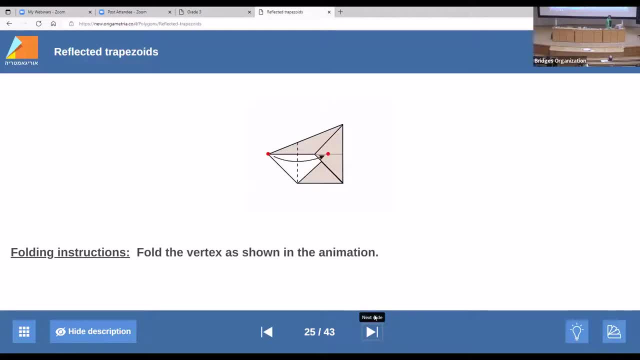 and they don't breathe because the reflex is to touch. And math teacher tell me I stopped to take the pencil and make write on the notebook of the student that I never understand why they do it. yeah, They usually don't have a understand it. 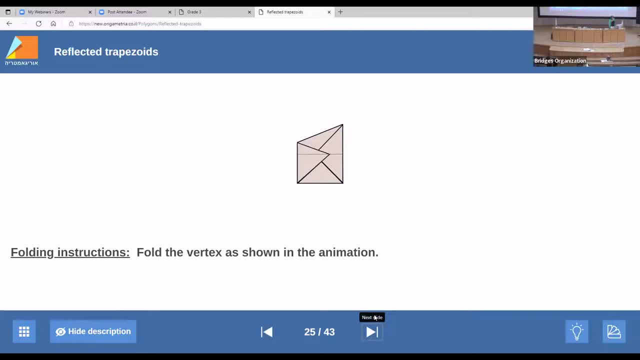 but after they experience that, they do it, But they find it's better to teach without. So after you got it we check again: is this how many parallel side we have? So we check with the measuring tool, okay, And we see that this side is parallel, two side parallel. 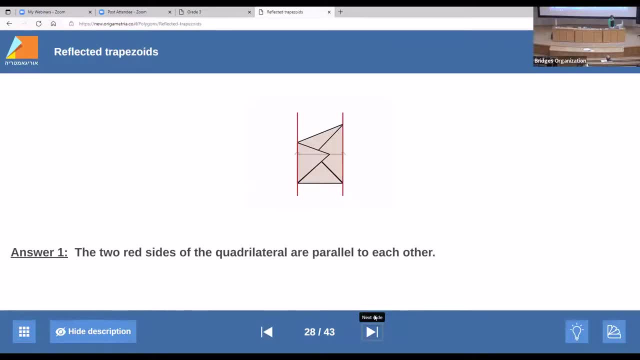 So this is how we mark it, And then we look at the other two side and we see they are not. So what do you think Is this trapezium? Now, the children know what is trapezium. they never forget. 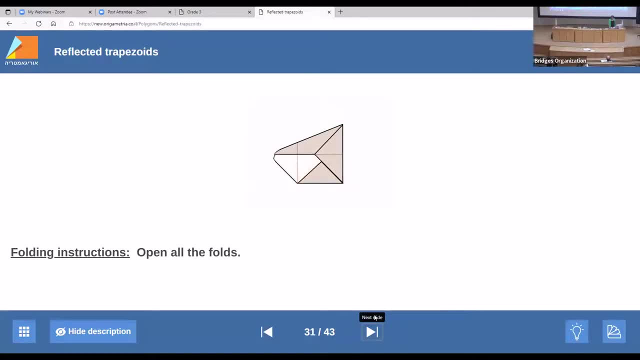 Okay, so now we open all the fold we make And this is very- this is one of my favorite part, because if you look at that, you find many trapezium. Some of them look like, some of them not look like. 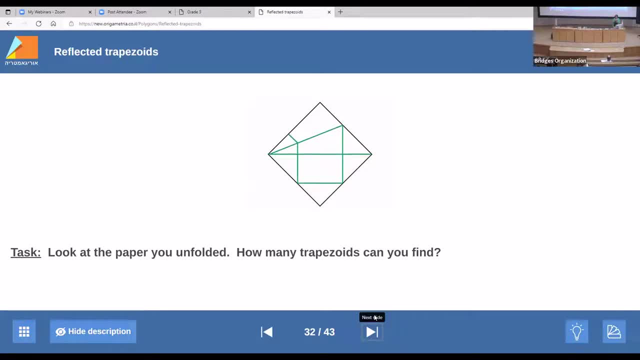 And when the child open it, try to find and find to discover. it's a lot of learning. Learning have to be by research, discovering. Yeah, not by what I tell you, It's by what you find, what you discover. 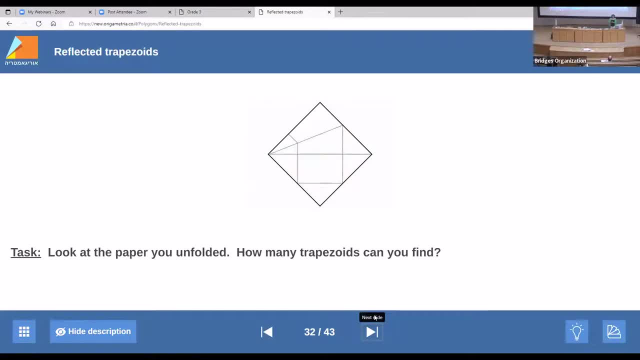 This is a learning. So now they can look at that and try to find out. And I never show them where is the trapezium here, Because I want them to go go home and think: is this more trapezium? 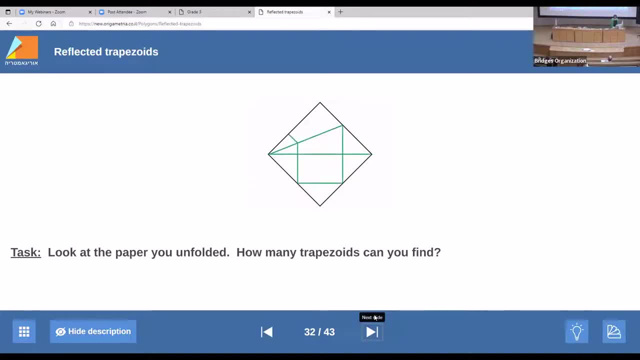 I want them to work Like. this student asked me a question. I never give them an answer. I always say it's very interesting. what do you think I like them to think, to think, to think. This is the most important. 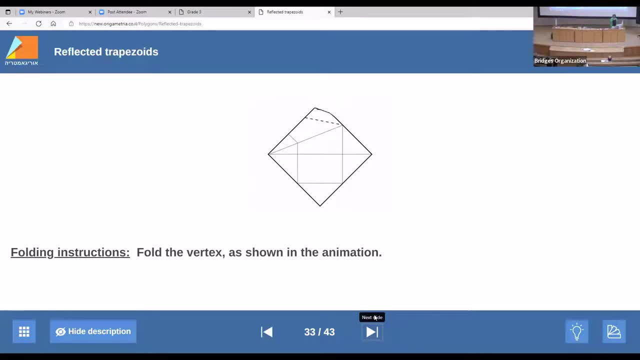 So now we continue to fold, but when we finish the fold you can open and look at it again. So look, make sure that you fold the vertex and it's showing the animation, okay. That's why it was important in the beginning. 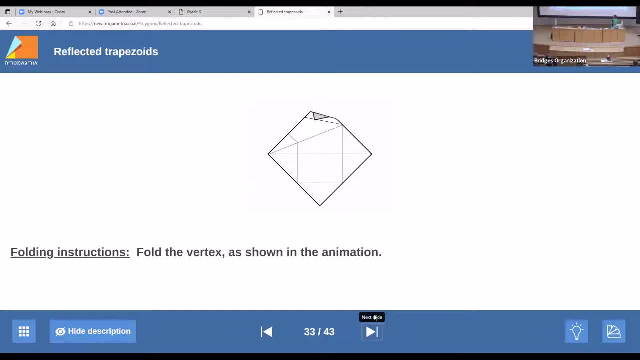 to fold in the same direction. Now, all the modeling, the augmented, are very simple, very beautiful. we'll create them And it's easy for the student to make them and for the teacher to teach them. The lesson, the geometry in the lesson. 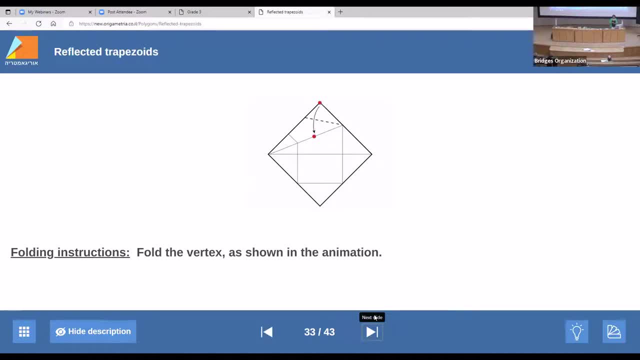 it's built with Dr Johnny Oberman, who writes is one of the writers of the curriculum. who writes is one of the writers of the curriculum. who writes is one of the writers of the curriculum in Matz in Israel. 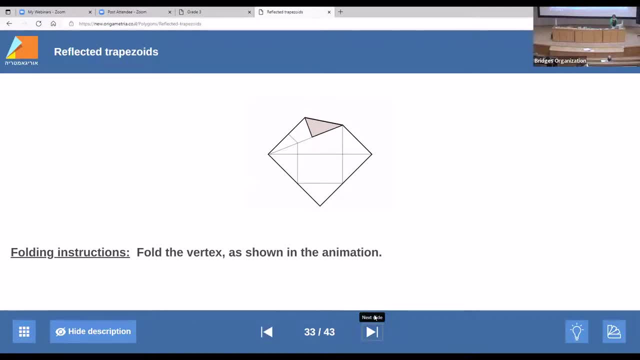 He have 60 years of experience And we put all of it in origami and I'm very proud of that. Okay, so now we fold. after you fold the small triangle, you fold all the triangle as it show. okay, Now, if you fold the triangle, 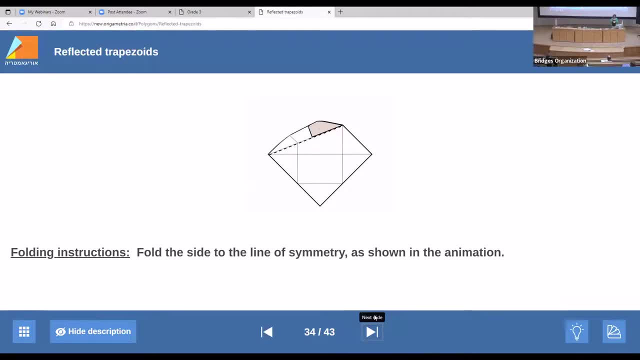 you fold the triangle as it show. okay, Now if children fold it and they need help, I don't touch a children's paper, but I come to him and I hold my paper in the same direction as his paper and show him with my 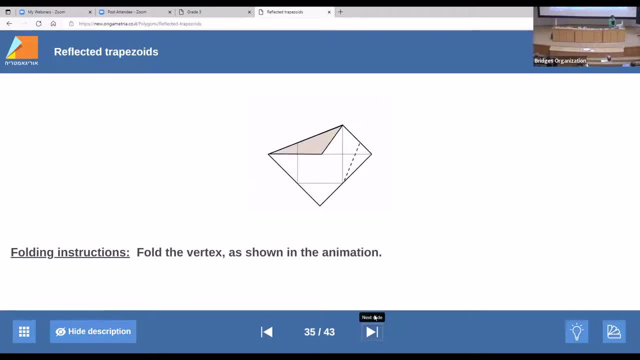 It's very important. Okay, so now I fold the side. You have a triangle and you fold the short side to the long side. So you see, all the lesson here is mathematics language. It's very important. And now we just close the small triangle. 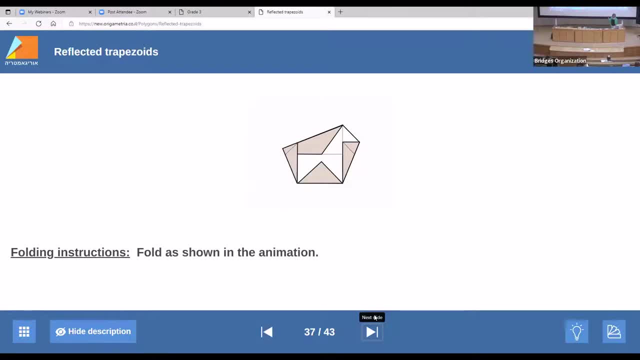 Do you know? you are the first people who see the origametry and you, You learn inside because we have another digital side And we soon- another two weeks- we launched a new one. This is the new one, So the first people in the world who see that. 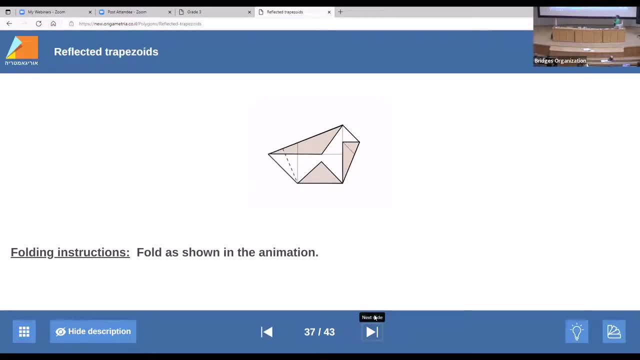 And today I came here And the first time I see it on the big screen, I got really excited. I put hours and hours, all my life I put in it. So now we fold the side to the line, As Joe And I we want to make to the Halls small tale. 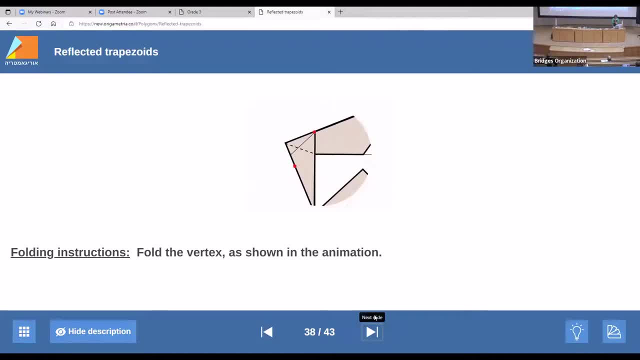 So we tell the small rechecks and we fold it, Hope everybody has a halls. So you see, At this point, And so you know, children are very creative And what we put here only small dot and a line. And I asked the student: can you design the horse? 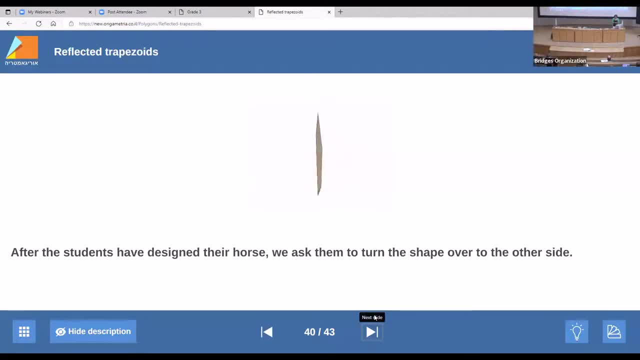 Can you put your own design on it And you can't believe what children can do. You know I did that. I'm not very good, But the children put a lot of beautiful design. So the most important I said to every adult: never draw on your work next to a children. 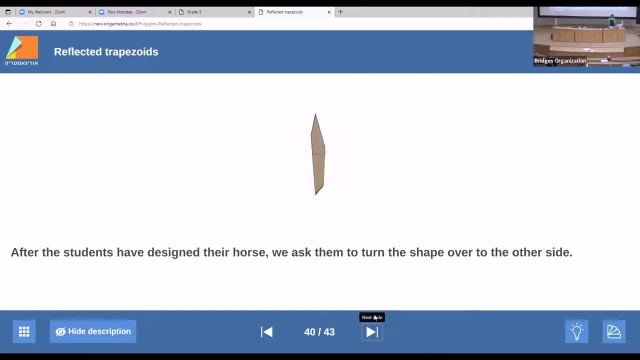 Never. If they ask me, I say to them I don't know how, And I put the crayon next to them and go And they draw. amazingly, I have a big collection of children drawing. It's incredible beautiful The way they draw, how they draw. it's just incredible. 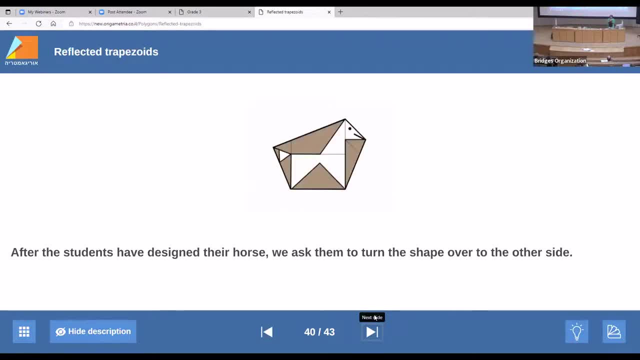 That's why, in this part, I want them to draw their own. So all the lesson the paper changed the shape And they say, ah, it's a butterfly, Ah, it's a frog. All the time they start to think what it is, what it is, what it is. 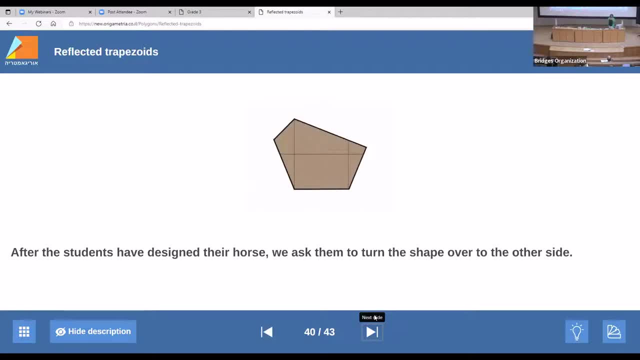 Because, origami, you tell them each step what to do. yeah, So how you be creative with origami? by not tell them what we're making. So they're all the time thinking what I'm making, what I'm making, And then they go, this horse. 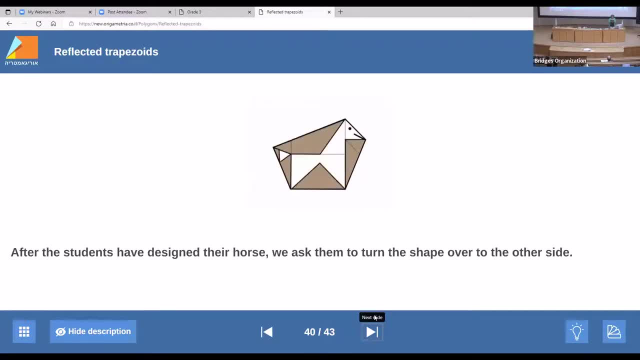 And now everybody can put his own touch to this horse. So if wait a minute, If you put a light, you can see the horse from the back. So if you look at the light, you see the horse. Just take picture of you. 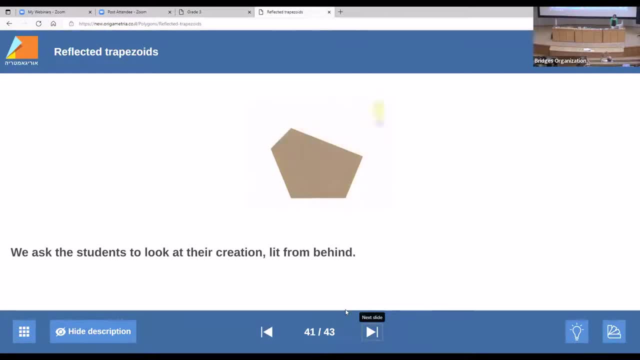 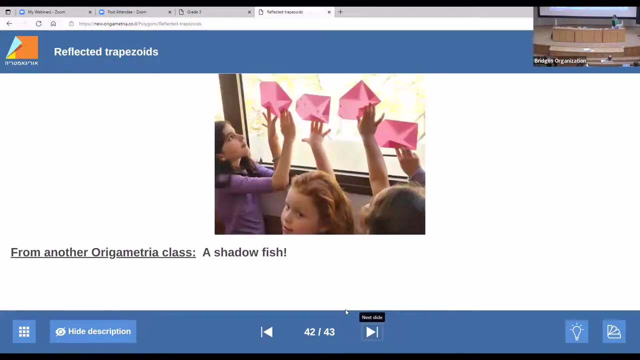 Where is Paul? Come from here. You see the horse. So if you design it, it will be more beautiful. So we did a similar model. It's a fish, And look what the children did. They'll run to the window and start to look at it from the window. 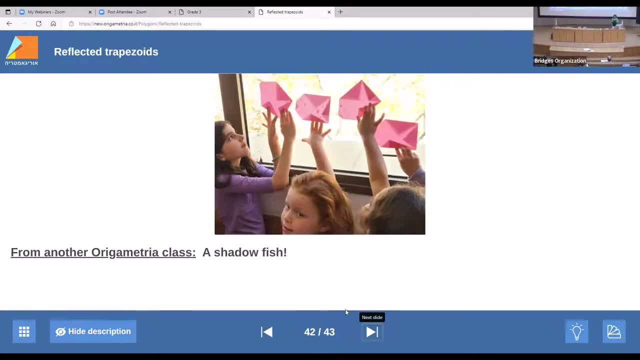 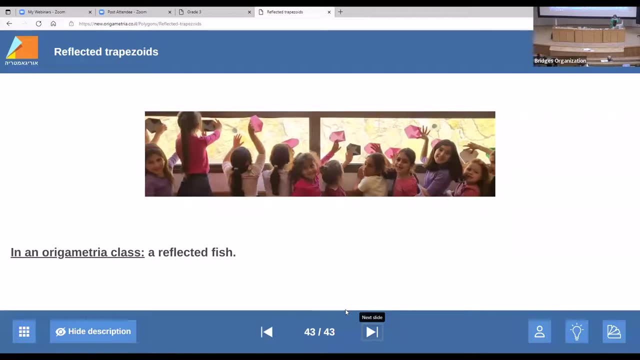 This is some of the teachers send me. They designed the fish and look at that from the window And this was just. they'll run to the window And it's beautiful to see it, yeah. So my question: did I teach them what is trapezium? 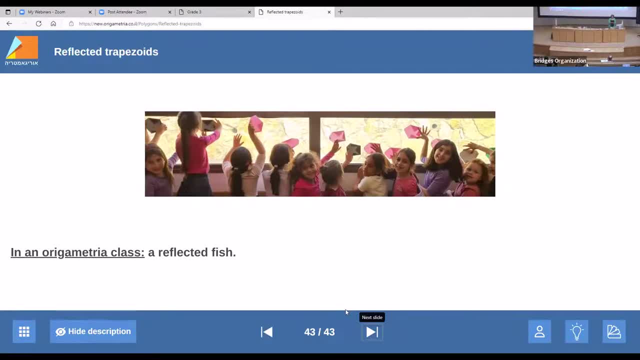 Did they ever forget that? And what did they learn? They learn to check, Yeah, And sometime the lesson finish and the children still investigate and learning and try to find it out. Um, the argument is from kindergarten to middle school. kindergarten, It's a bit different, but it's beautiful. 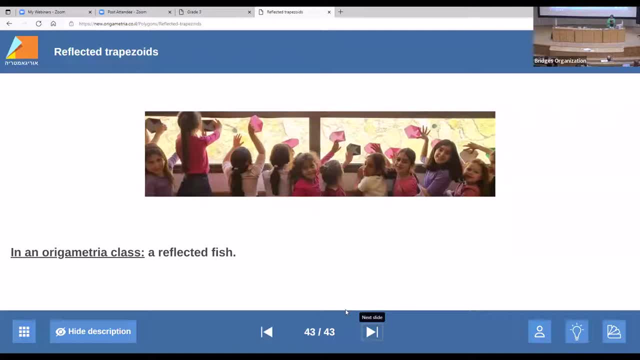 And one of the kindergarten Teachers say to me that one of the kids who's not participate and not very active, Uh, the move to a new house. So they went to the new house, house empty, and the kids run to the living room and look and say, look, mommy, it's a lot of square here. 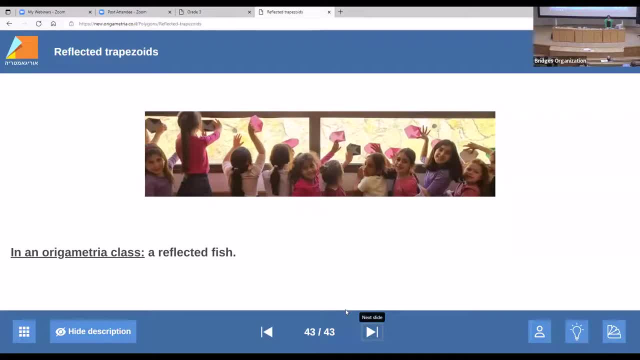 Look, this is the the the right angle, and start to run around the house and just look at the tie. It doesn't look at the room anything because what we did, we play with them. It Geo Metry. 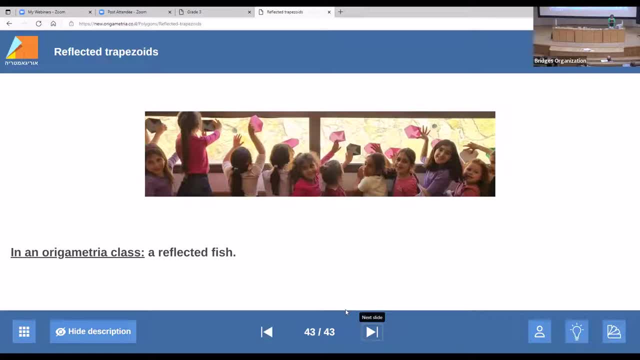 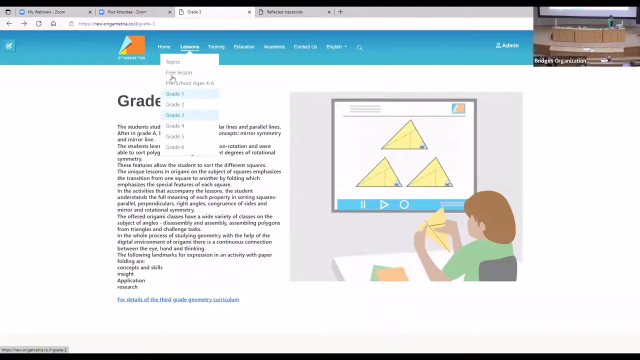 So the geometry is interesting and it is- it's the most excitement, I think- topics. So after I show you what is origami to a lesson, I can talk to you about origami. So I go back. Okay, This one. 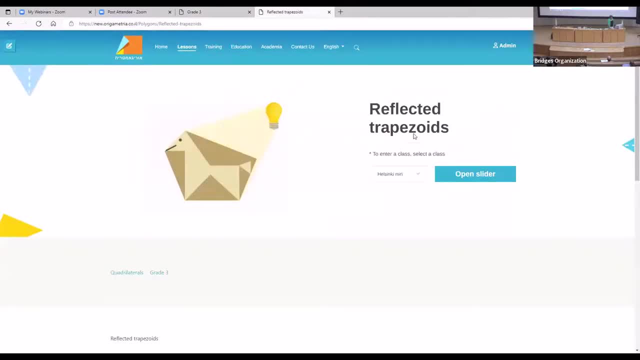 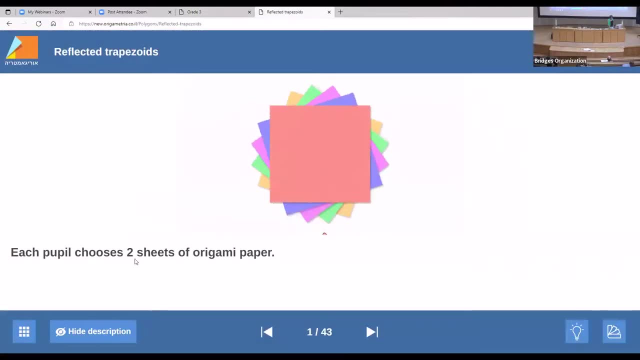 I go From here, So I close the lesson. by the way, I need to show you something. Um, if the teacher want to see all the step, she can press here and she can see and go to a certain step. She won't. if she want to hide the text, she can press and the text will go. if she doesn't like the blue and she want to orange, she can change the color. 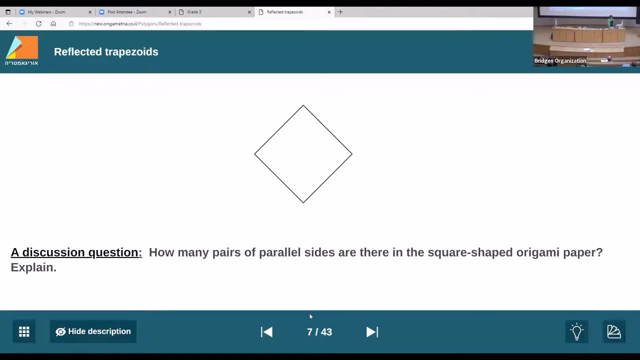 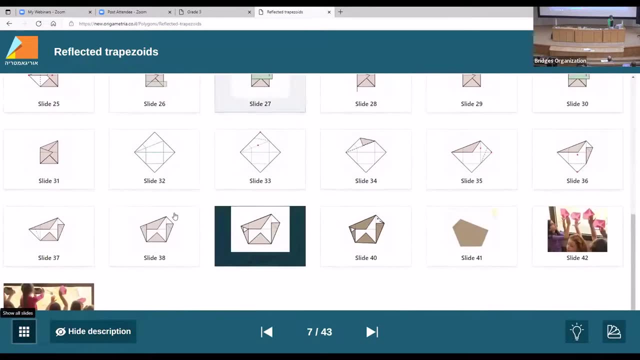 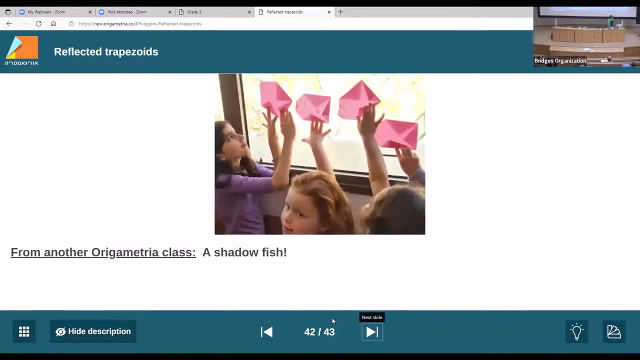 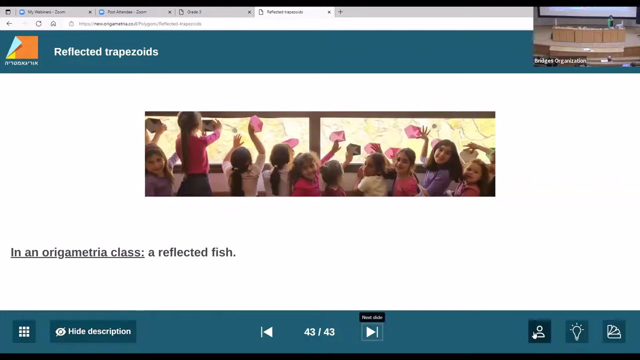 Yeah, She can change the color. Yep, When she finished to teach the lesson, Let me show you here: Go to the end, Almost to the end, Um, usually in the end I. uh, here it is. You see the teacher drawing so she can go to her area. 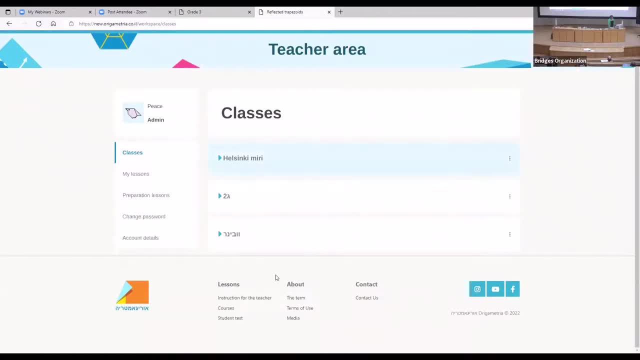 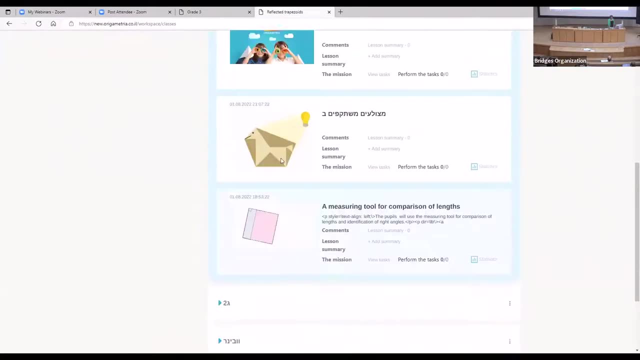 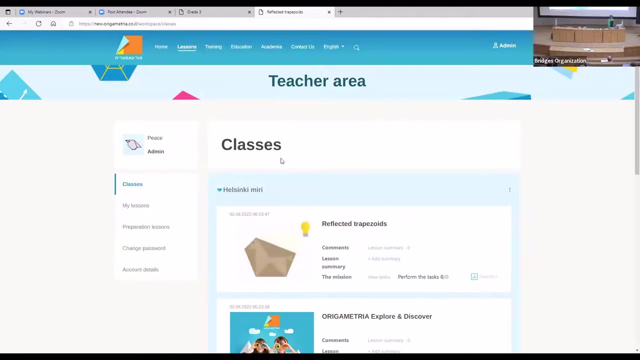 And all the school. She is all the classes she teach. it's here. if she press on it she find all the lessons she check. also she can send um some quiz to the student after she teach. so they need to answer that and then by the answer she know if they understand the topic. but in the end of the quiz they have 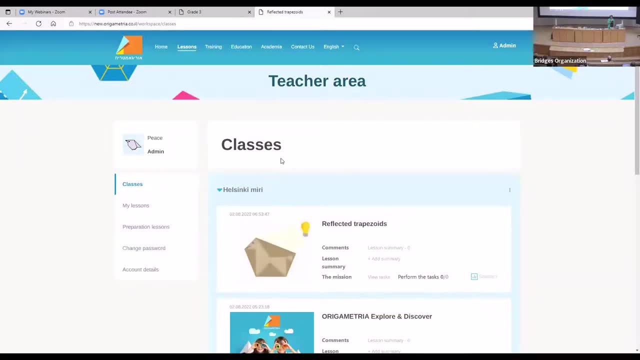 the step of the folding we did because the children doesn't want to go home and just answer question. they want to make the holes we make today so they have motivation to go in. so if she want to go in student, want to go in, they can go to student area. 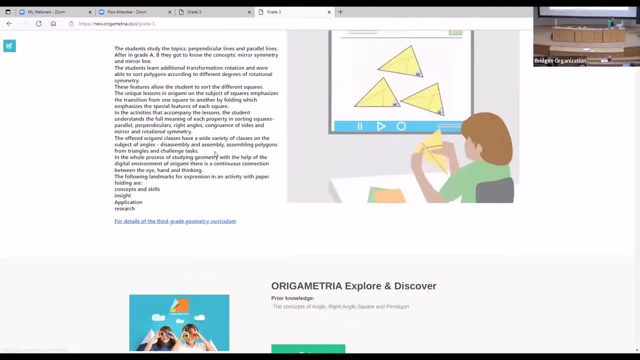 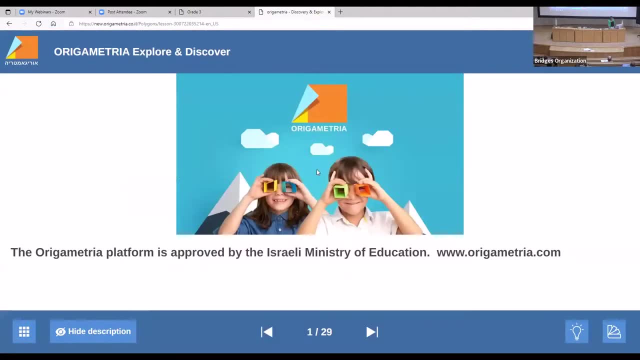 so i'll go back to third grade and i talk about now. i can talk about origami, okay. so origami is approved by the education ministry in israel as a part of the curriculum and we have about 160 000 students who study every year. we have more than 600 school 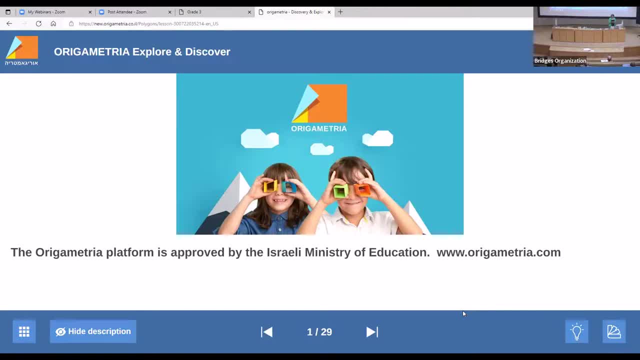 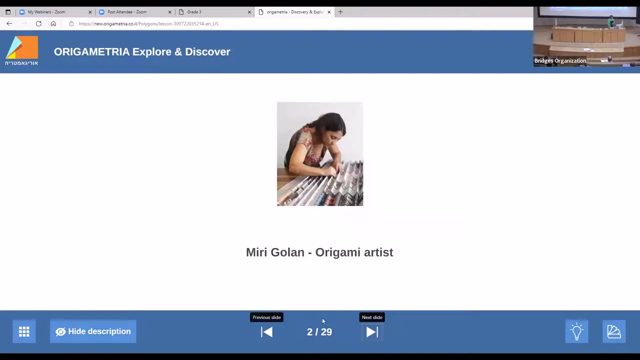 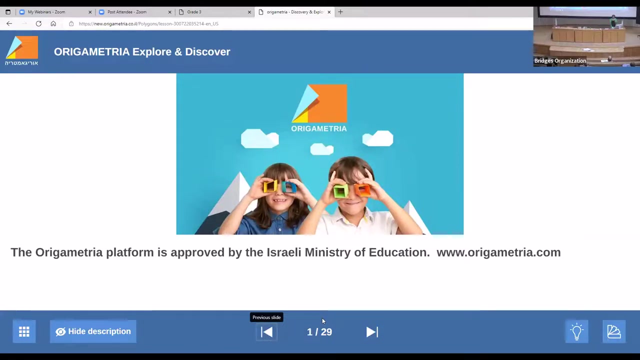 and it's the four years the school renew the uh membership in the site. we usually sell them membership for for one year. um, if you go on the online, you don't see this one, you see the old origami site and after three, two, three weeks you get a new one. but the old one is beautiful too. 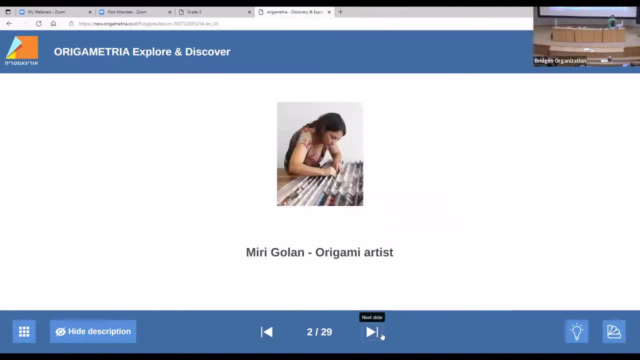 i have to say, um so who i am. i born in jerusalem in israel, grew up in jerusalem. when i do art, i'm an origami artist. when i do art come from my region, from the way i live, the way i grew up in jerusalem. 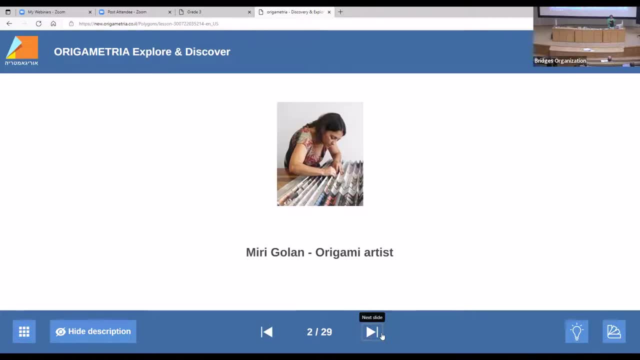 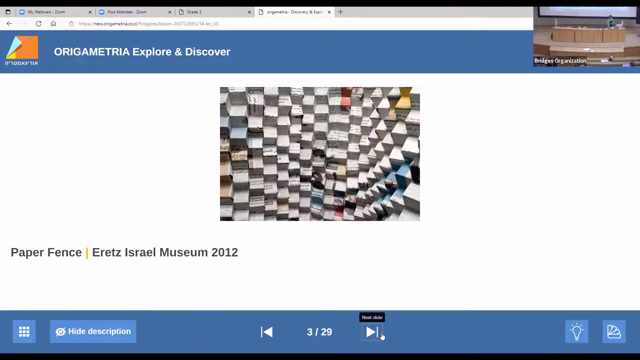 since established the origami center. we work with israel in palestinian, israeli, arab. we work with all kind of population in israel. um, this is a artwork that i did on a newspaper- one side arabic, one side hebrew- and it was in a museum and i called it paper fence. 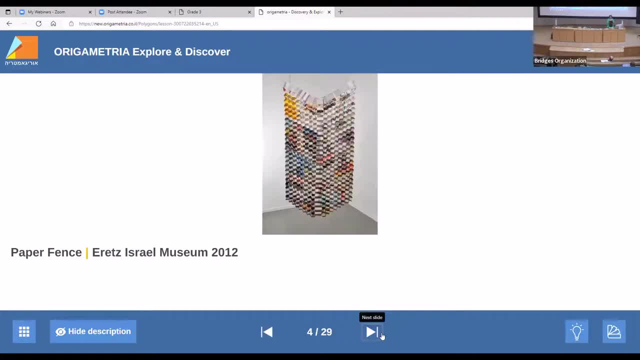 and sometimes i use to stay there and people didn't know i make the work and i like to hear what people talk and some people say it's so nice when the arab and jewish together the language and some people say, wow, it's really once against each other. 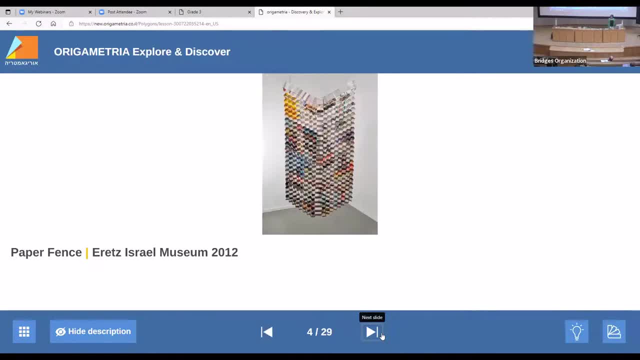 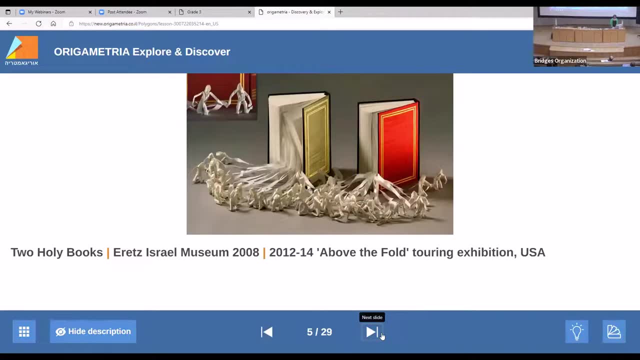 so it depends what their opinions are. that's like what they think about my work. i like it. uh, this is two holy book, um, and from the holy book i cut the paper. it's a handmade, not text, and, please understand, it's still in aありがとうございます, so i'll let you know earlier on how they're called. 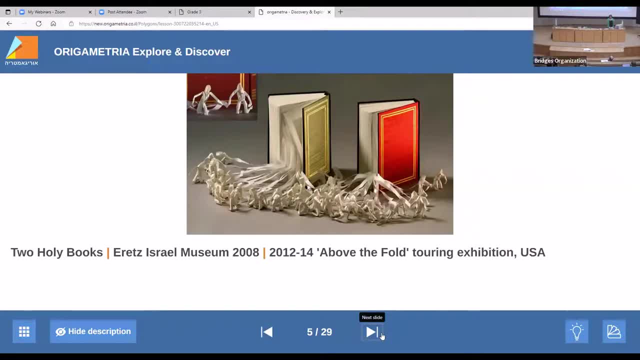 on it because the word is word of God. so I don't put text and I cut the paper and make for the men from there. but the men is still connecting to the book but you cannot know which men belong to which book. this is the two men who's coming from the whole book. it's a. 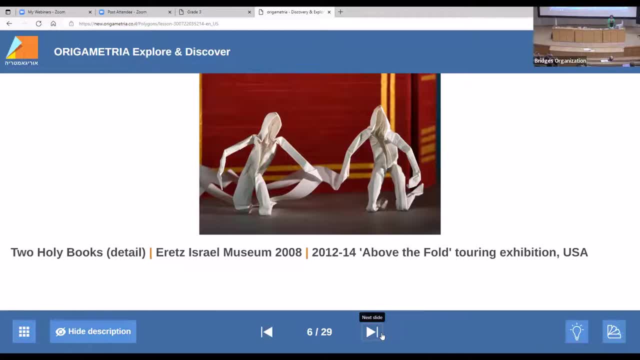 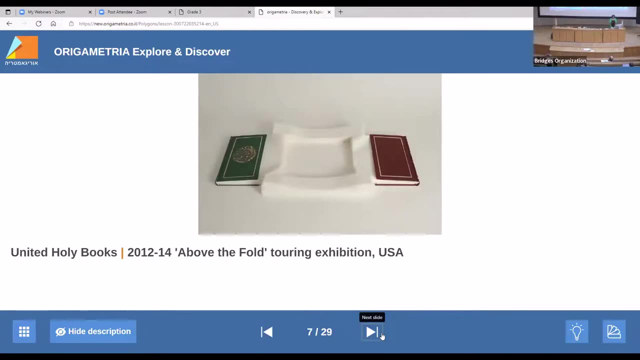 exhibit in the museum in Israel and been in, I think, 14 museum around America for five years, and now it's in the museum in South America. this is another two holy book. um, this is actually one sheet I like to fold from a bible paper. um, I like the touch and it's very special and it's cut. the same sheet moved to one. 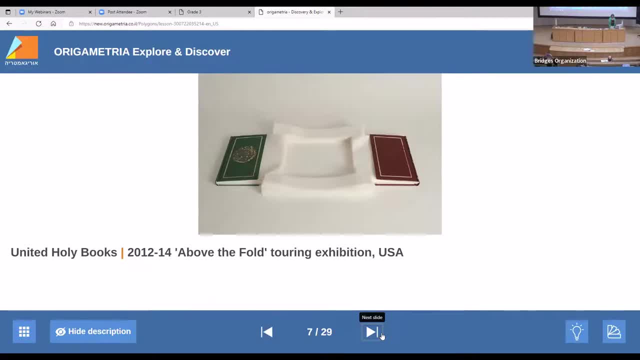 um and another book and just show the connection between the two books: two different holy book. this is my favorite work. um, this is the Torah, the Jewish Torah. usually it's in the synagogue, it's closed in the cavern, but in the middle it's not twist, it's straight. now the two rolls made. 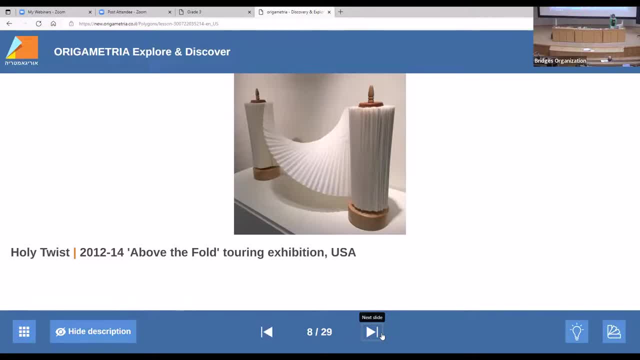 from a bible paper but I bind handmade binding one. while I fold it it starts to be a circle. the middle is the same material. they make the bible from a leather of a cow, but I twist it and this is my way of saying that you twist the religion, or 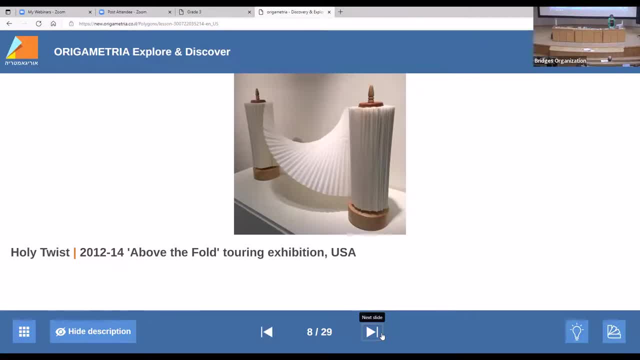 um, but many times you've been to 14 museum and many times I've been invited twice to open exhibition with that. it was part of origami exhibition. Paul exhibited it too, And I like to see the comment of the people how they think. 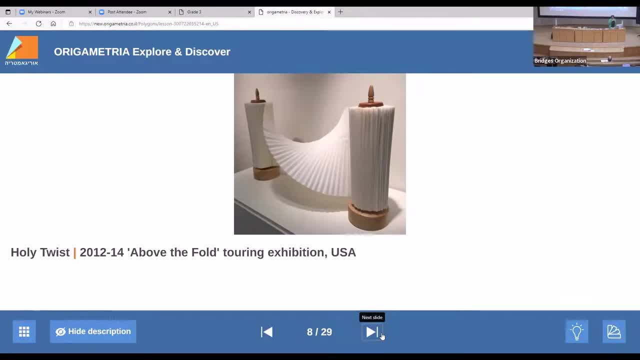 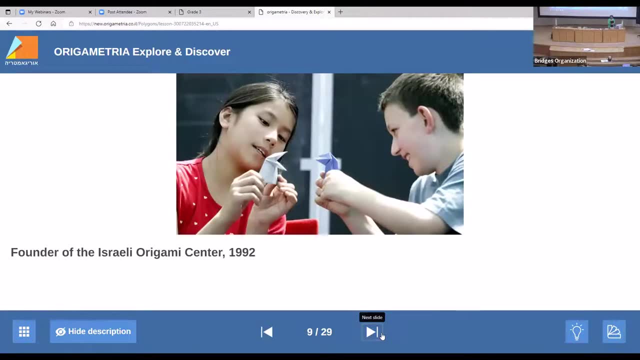 I like them to think about it because this topic is burned inside me and I grew up in Jerusalem, So in 92, I established the Origami Center. People didn't know what is origami in Israel and I started to spread it around. 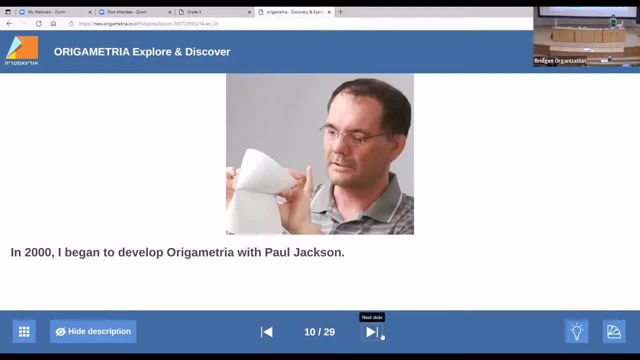 And in 2000, I went to origami convention in Germany and I met Paul Jackson and we got married. five months after He asked me to marry him by making an origami ring from half a dollar butterfly ring. So we worked together. 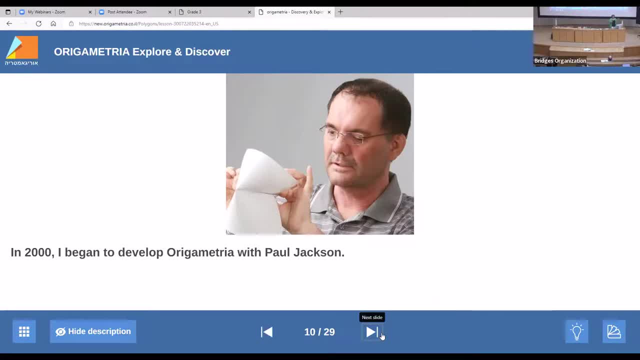 We have two different areas. You'll hear about him soon, But we also have working together and he do a lot of work. He do a lot of work for origamitria. This is Dr Johnny Oberman. I feel privileged that I'm working with him. 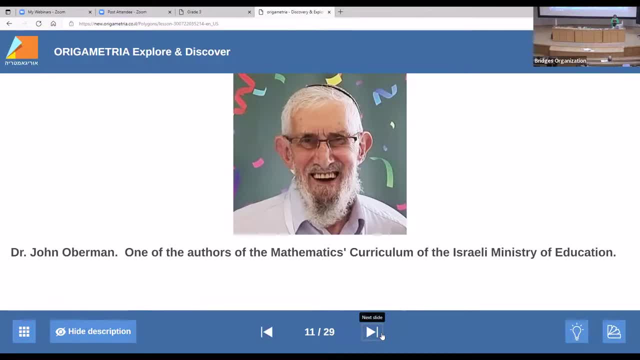 because he has 60 years of understanding and develop curriculum in a maths education And he develop origamitria with me. We working together And I feel I put in origamitria Dr Johnny Oberman legacy of the geometry learning because he look at origamitria. 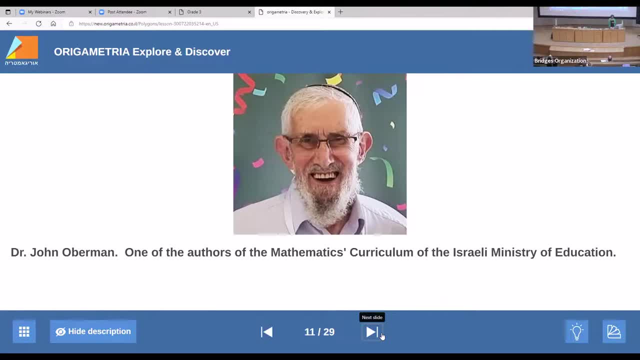 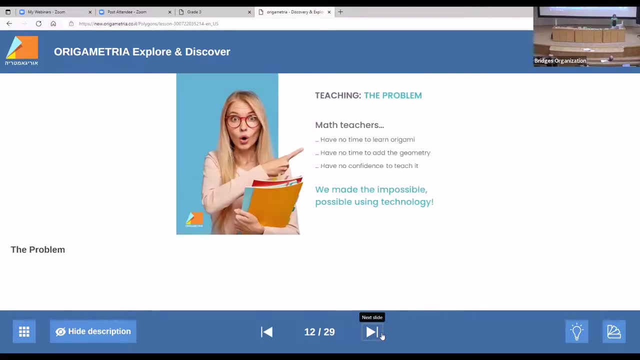 and look on the geometry from the eyes of the student is very important. But many people who's doing origami say I try to convince the origami is good and all the time get a comment Now. so it is a problem because the maths teacher 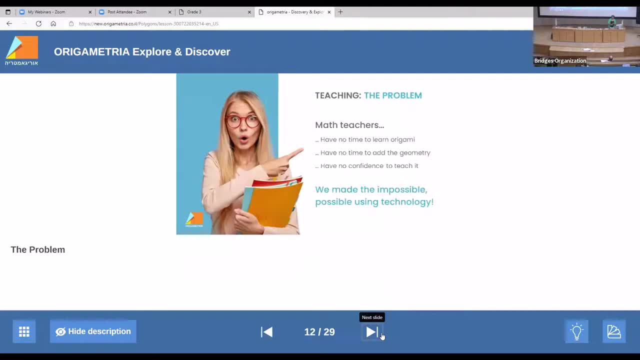 very, very busy. They don't have time to start to study origami. They don't have confidence to teach origami. And yes, origami is a good tool to teach geometry, But how, Yeah, so how we can make the maths teacher to teach. 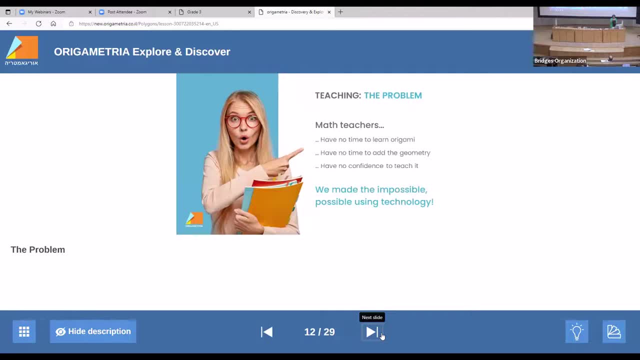 So in the beginning I develop a program we call origami to develop a learning skill. I teach in a special education school for 20 years And there's I develop all my teaching method. They are very unique, So understand, the teacher doesn't have time for origami. 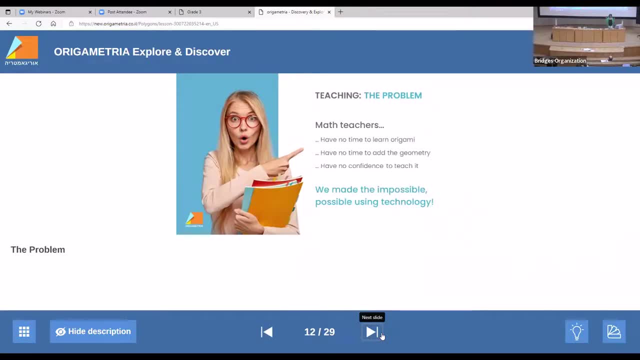 But, as I saw, I show you the lesson. you understand She doesn't. if she wants, she can go into the lesson put her own comment, but she doesn't have to. She just can come to the class, screen it and teach it. 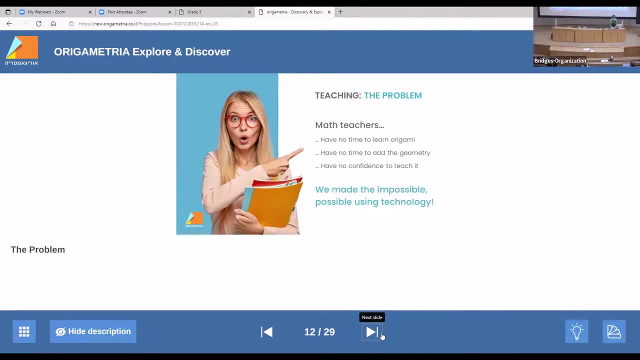 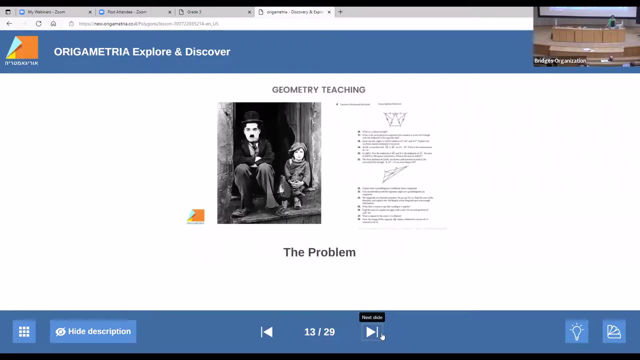 And part of the problem that the teacher bring all this misconception to the children And while she teach with that we make sure that she's accurate of the teaching And in maths it's important. So also another problem with the origami teaching geometry. 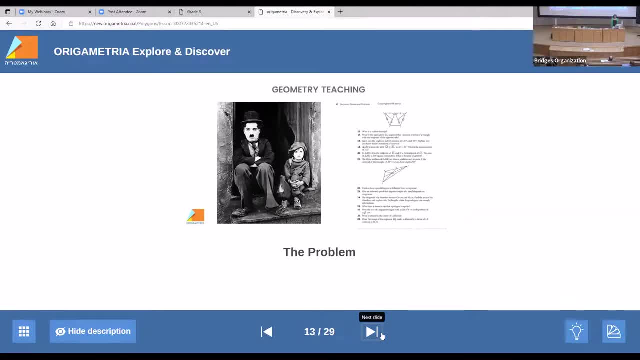 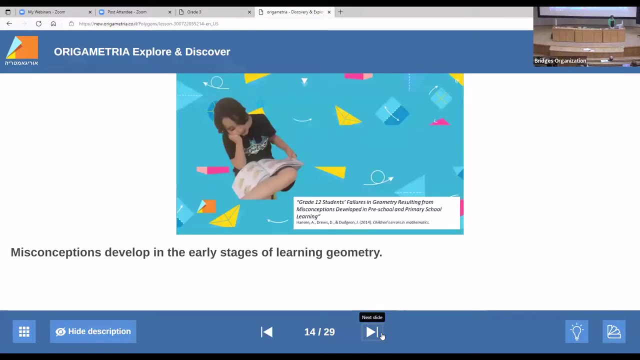 is. it's impossible. Even they try to put animation and something fun, it stay on the board. And also they still use books and the way they teach geometries makes geometry boring and geometry is excitement topics. So part of the problem: the misconception of the student. I'll give you example. 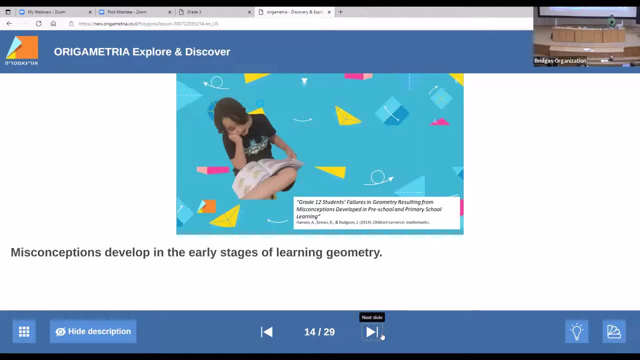 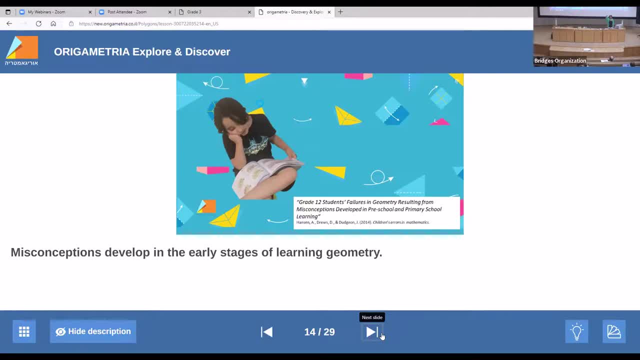 One of the student. tell to the teacher: if you hold the triangle like that is a right angle triangle, but like that it's not. If you go to the class and you ask the student what's that? The students say it's a square. 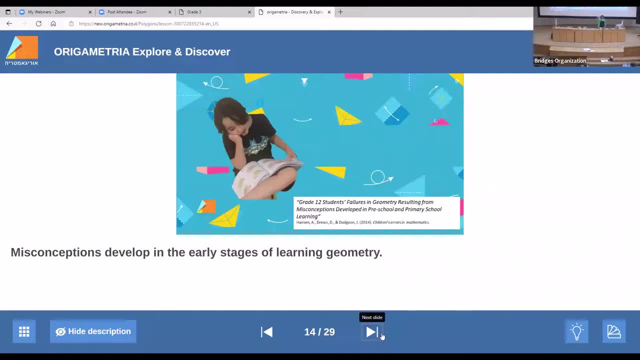 What's that? It's not a square, It's a rhombus. how i change it? it's very nice. i said to them: okay, why is this? well, because i have an equal side for equal side, have right and again, and i check it with the measuring. okay, now we move it. 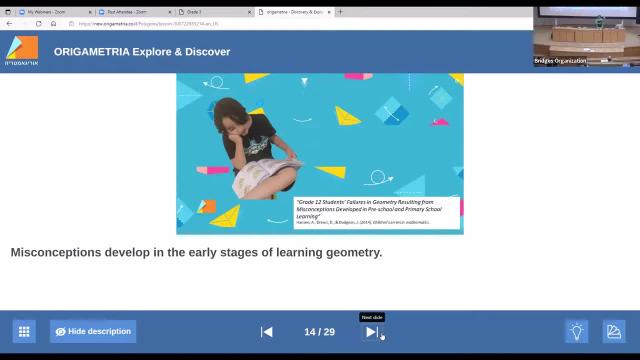 like that is anything of the square character, of the square change. let's try. is it still have equal side, still have the right angle? so my name is miri. when i sit, my name is miri. if i turn to the other side, i still say, really, and that's it, it's gone. they know and they understand, it's so. 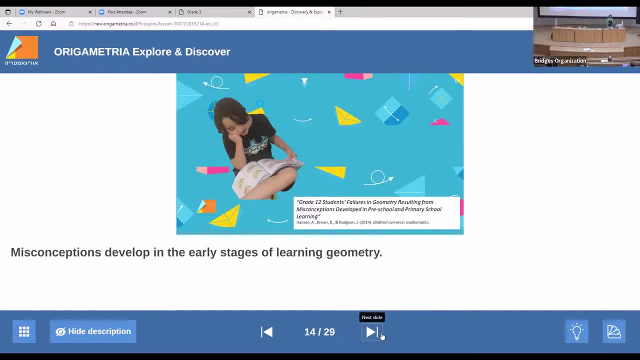 the misconception. it's a big topic. it's part of the reason that the student fell in the exam. now you have to understand. many people- and i know there's many, many foundations- put a lot of money in middle and high school in to improve the geometry, but the problem is not there. the problem it's in the kindergarten. 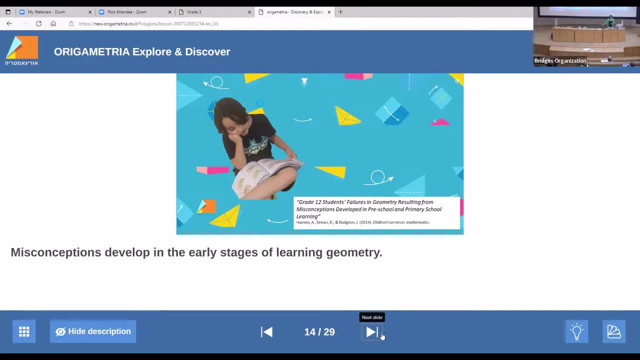 we need to start with the geometry early age. foible start when i was four and i do believe you need to start four years old to see geometry. if you teach good geometry in the early age, they have no problem with the growth, because to understand geometry we need also a good imagination. 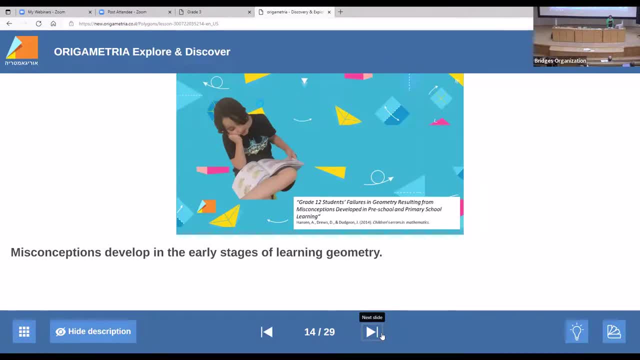 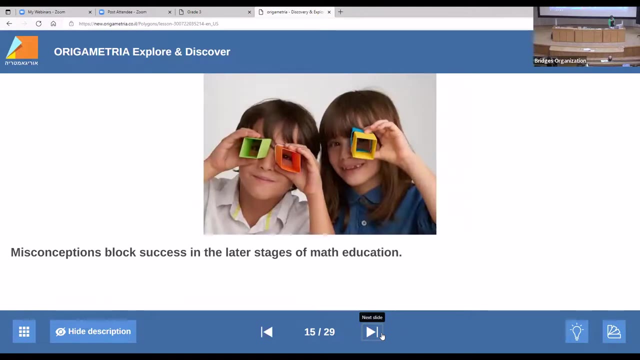 and and when you do it when you're young, then it's much easy for you. if you talk to kids four, five, six, they have really amazing imagination. it's helped to understand the geometry. so i give you example: um, this triangle. this is a research who have done tel aviv university. 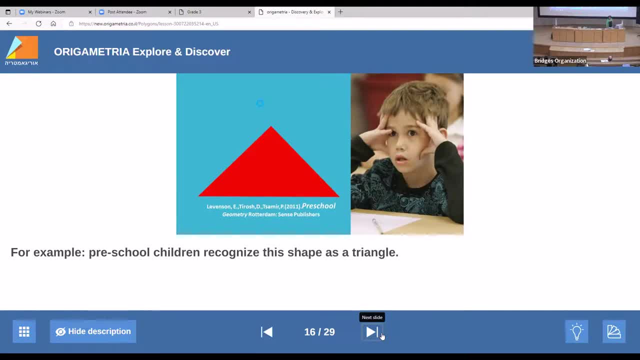 i think, um, so they show this to this the children, kindergarten. if you have children about four, five, even six, ask them what's that? they say it's a triangle. why? because always they showed in the triangle like that. and now you ask them: is this a triangle? 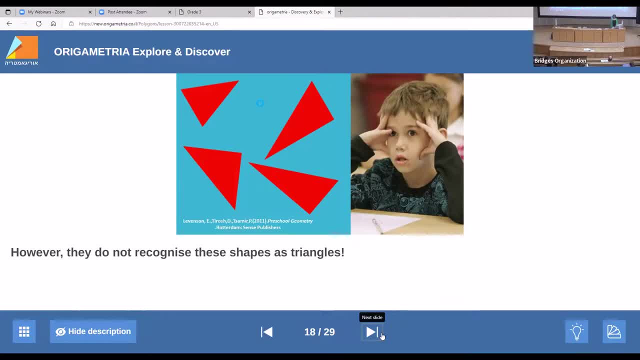 or even you show them like that, they say no, it's not. because all the time they show them like that them the same shape of a triangle, it's all the time like that. so if it's all the time like that and you move it, they say it's not, but how we teach them in the regular matter we say okay. 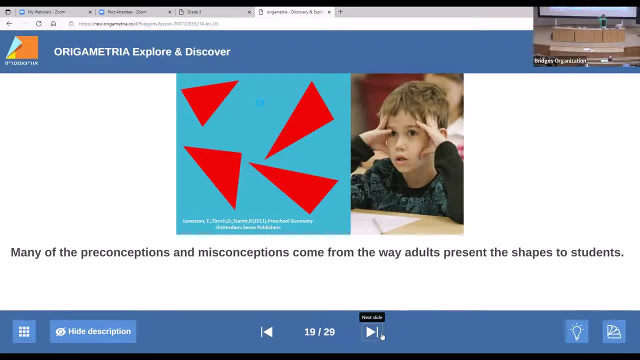 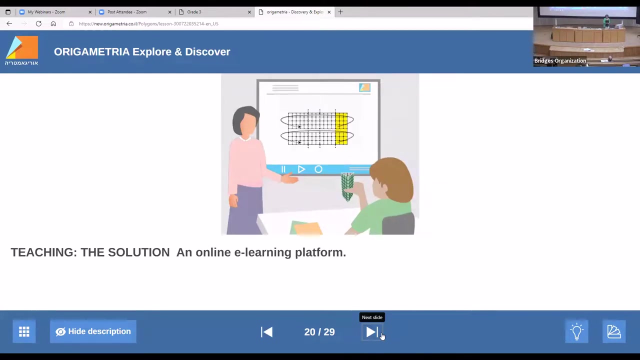 we don't ask them if this is a triangle. we ask them: can you count how many sides you have, how many vertices you have? then you know they understand the shape by investigate, the shame, but not by memorize. so, of course, the solution for all this misconception, it's the origami online. 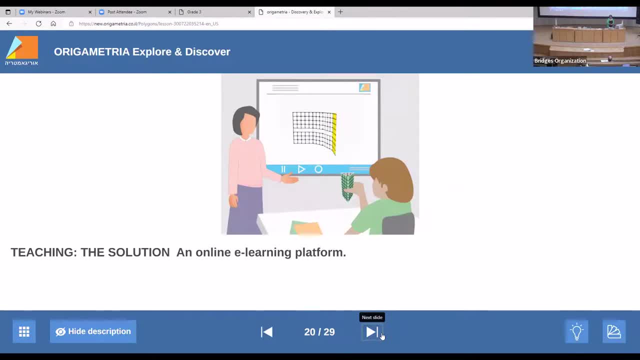 it's easy to use, very friendly and also make sure the misconception doesn't go, because we are the teacher of do it. um, i did with the dr johnny oberman. i trained a lot of maths teacher and we asked them: what, how, what is the definition of an angle, how you do it, what is the definition? 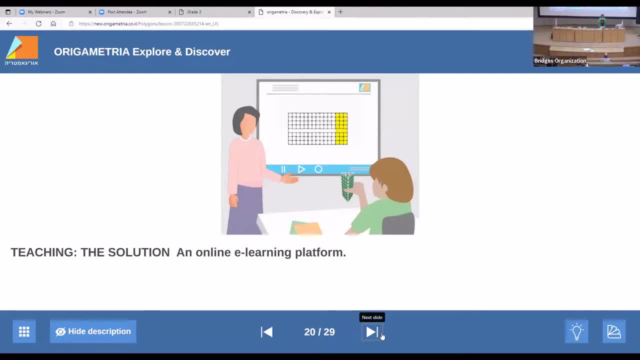 and the way they explained it. you see in the in the pizza exam, the result: yeah, they say it's a corner. two line come out from the corner. okay, so the children say the length of the angle is the angle, or maybe the distance, but angle it's the distance between one to another. 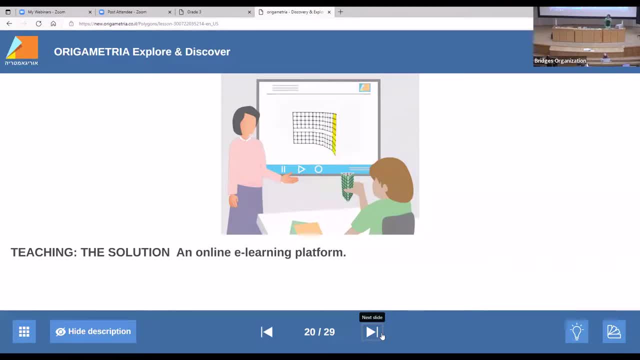 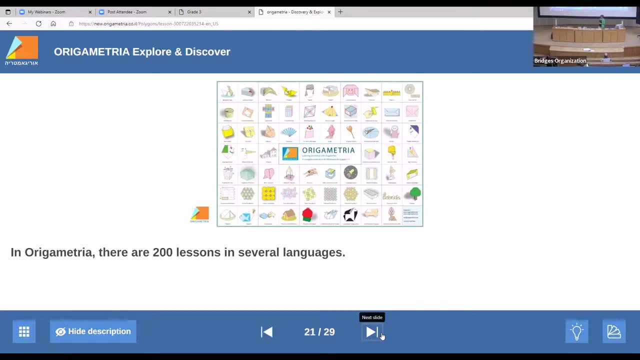 so when we do it with our origami it's much easy to escape all this misconception. so we have over 200 lessons. each model here teach some topics and it's attached to the curriculum in math. and actually all the curriculum in education all over the world is the same. i've been teaching in many, many countries and i know it's the same, so 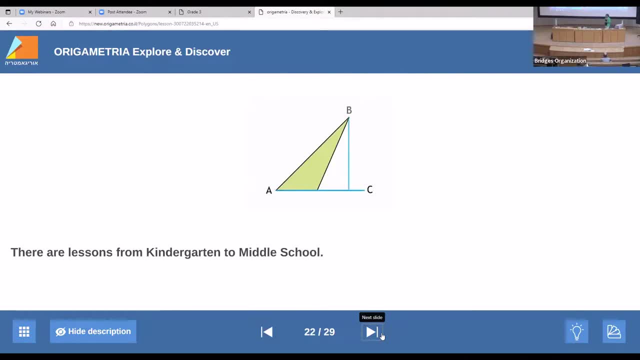 so we have 200 lessons in each one teach different topics from kindergarten to seventh grade, like this one: they make a finger, uh um, nail, and they learned about the height of a triangle. or here, to do tiling. it's a fifth grade usually. so the fold and make this styling beautiful lesson, this one or this kind of tiling. 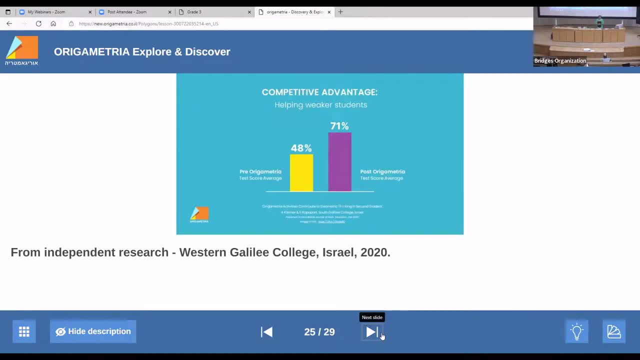 so i've been asked by one of the professor to go to school and teach their with her. in the beginning she was very negative: what i'm doing with this origami, i'm a math person and all this. so we did teach and she saw what happened to the student. she saw the knowledge. 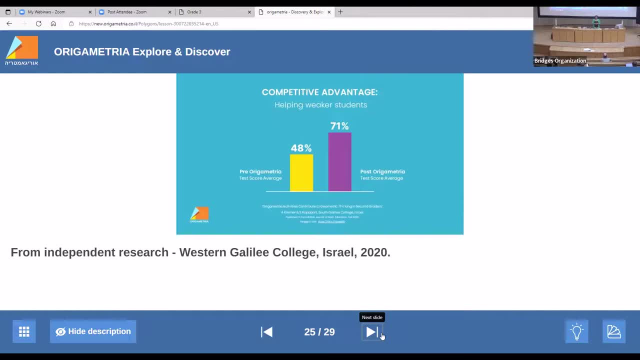 then she did the research about origametry and she wrote a few articles about origametry. so what she did, she just did it before covid. she took the weak group and strong group. the control group was a strong group- it was about 71 percent- and the weak group 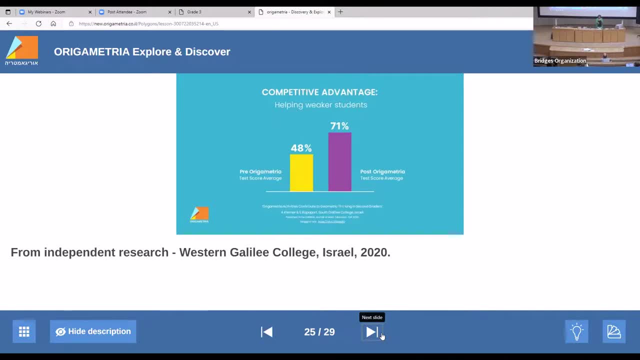 was about 48 percent. she used few population- arabs and jewish- and she saw after a very short time the weak group have the same result as a strong group by study with origametry. so it reduced the gap between the strong and the weak and we know. 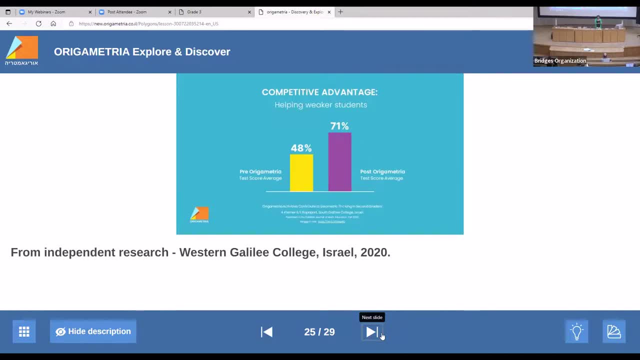 after covid this is a very strong topic because the strong people can manage, can take private teacher can, but a week don't. so i know this year is going to be another few research about origami i've been asking. of course i have nothing to do with this research, they do independently. 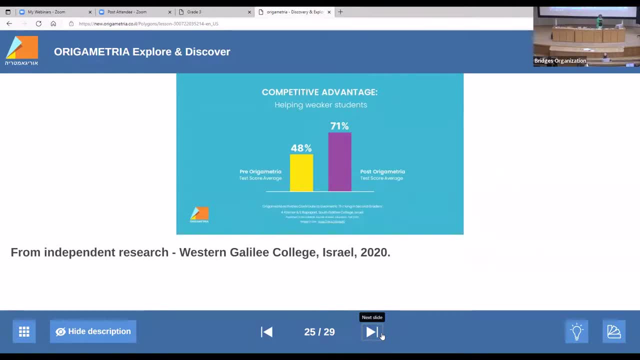 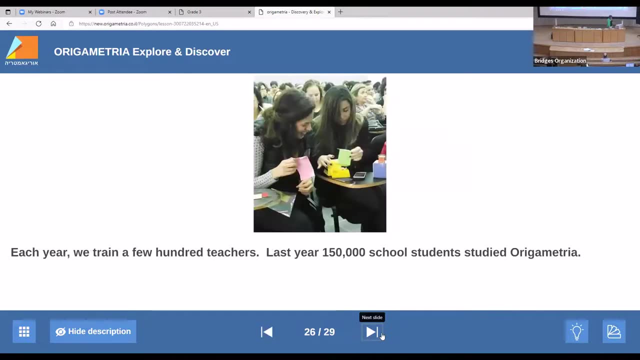 and even the college buy the membership for the origami and do the research. every year i trained um hundreds of maths teacher. it's nice. in the last year i don't need to drive anywhere, i just do it by zoom. before i used to take the train few hours to here, to here and it 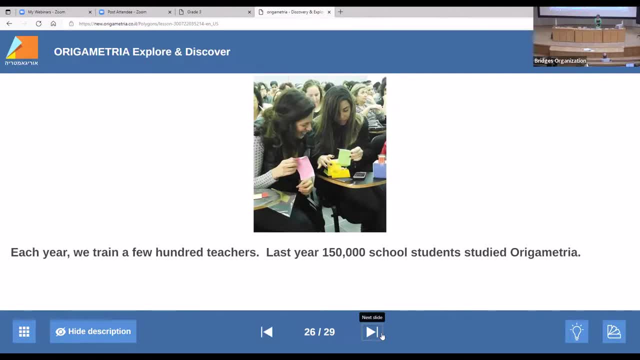 was all the time on the road, but now i do everything by zoom. it's nice. so we train a lot of maths teacher. um, we don't train them because to to use origameta e-learning site is very easy enough: one meeting and they know how to use it. but also we work with them about the geometry. 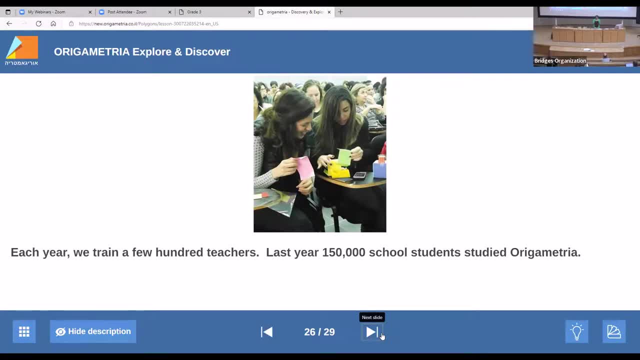 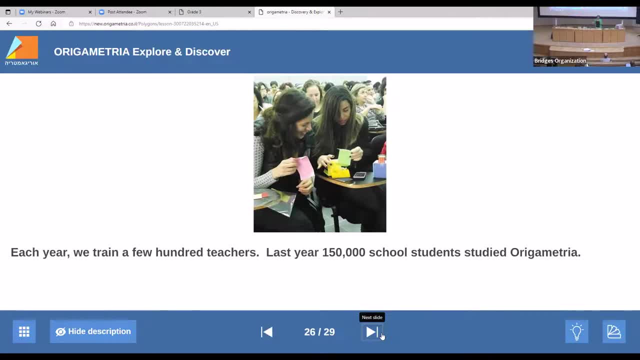 i'm proud of that, you can believe. i woke up in the morning and that's what i do. all right, all right. lesson with dr johnny oberman, developed with paul the models, and i just leave that and i put all the lesson and work in it. i just eat and live and breathe this. i look at the, i look. 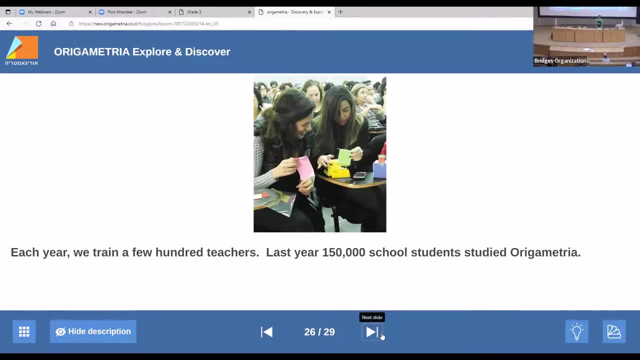 at the origami as a work of my life. come on, bring me my best husband. you know i want but. but origami it's amazing, amazing tool, but if we use it not from the origami side, from the education, because sometimes origami people come with the excitement and they need how to excitement and teach it. and i came from the point of the. 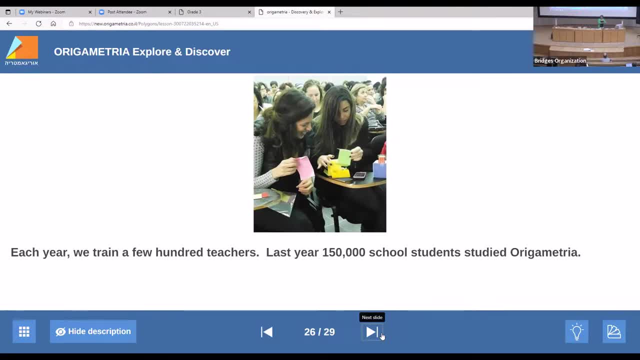 education ministry needs what the student needs, what the system need to make the student better learning and joy. because in the beginning, when i came to the education ministry and i said: look the children happy when they study, happy, it's smart. they need to learn what's happy. 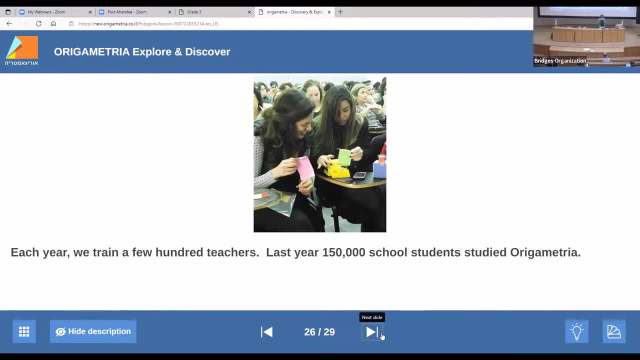 um. so the joy is very, very important. i'm not talking about the motor skill, uh, space awareness and all the other learning skill that when i was starting with origami i was really um emphasized it. i don't emphasize them because it's in plant, in origameteria. 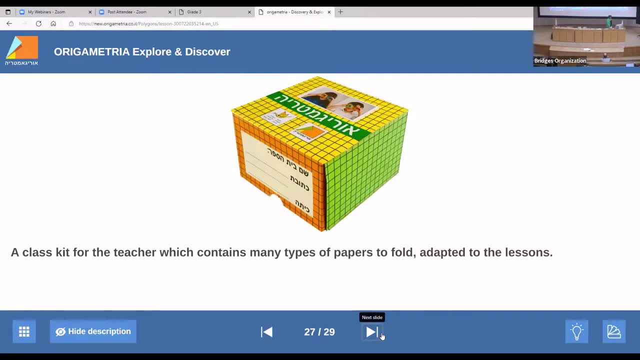 so what you see here, you got paper for me. yeah, the paper you get, we print them in israel. i refuse to buy paper from china or from other places. we print them in israel and the people who pack the paper. it's a handicap, um, and it's very important to me because it gives them work. 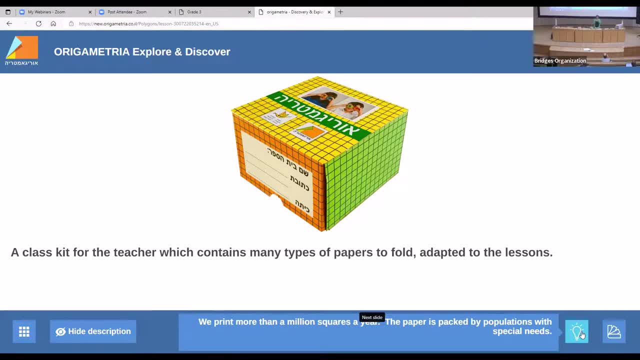 many times i go to the place they are packing our paper and i'm very happy that i woke up in the morning and they have something to do like packing our paper. so every teacher or every school who buy it, who buy, pack like that with this paper. some of 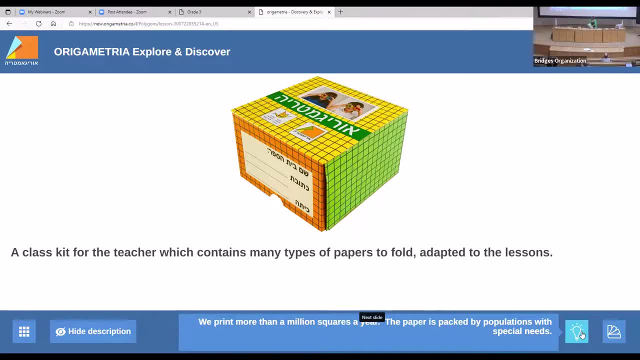 the paper. it's a paper like if i want to teach just a minute, if i want to teach the children measuring, so we have a special paper that each square it's one centimeter, so they can learn that you know this. um, if i take two paper, put it on each other. they're equal. and now i fold to a triangle. 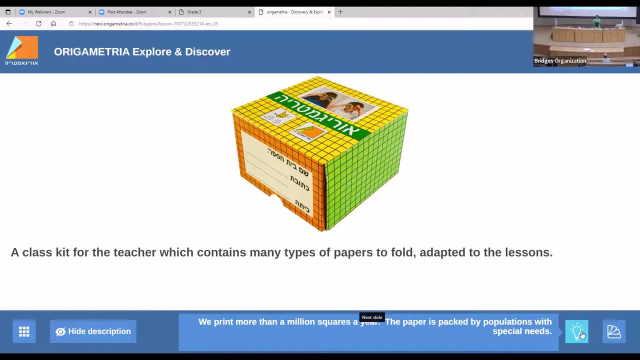 and i fold this one to rectangle and i ask them: is this area equal to this area? no, they're different shape. yeah, but when the c they are the same. i rotate them and you can see: and this is a half of the same square and this is a half of the same square. then we know they are equal. even it's two shape. so we have 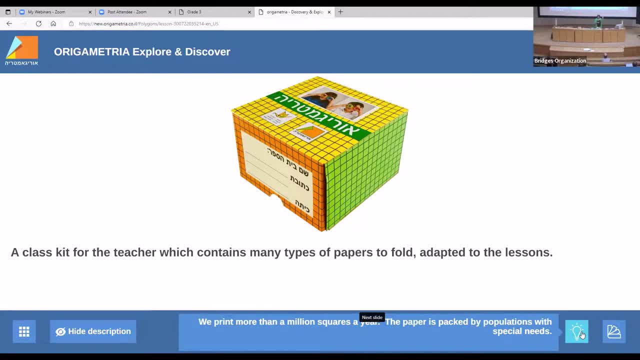 a lot of lesson with the square paper that we do three different uh size, but they are equal area and then the children understand it. we also have special paper with a dot or as a metric so they can um, build and work out how to measure with that. so this spot come. 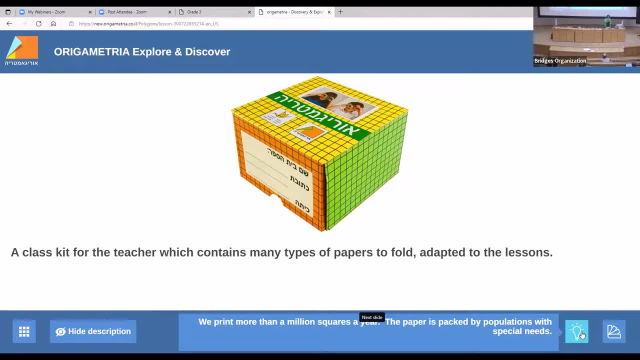 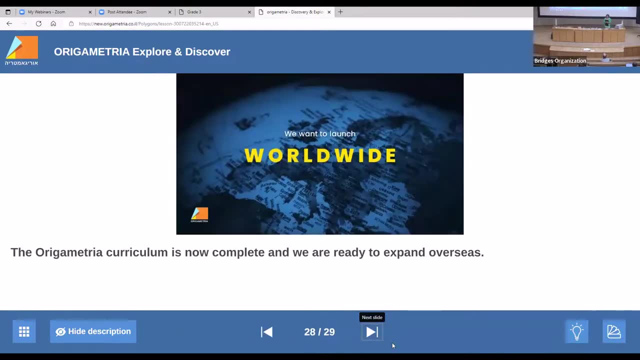 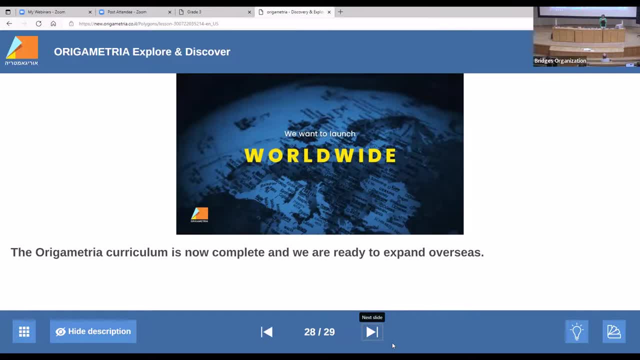 please let us know because, uh, in a new, uh digital, um argument- e-learning site, we can have any language easily, very easy to turn it to any language, and we do believe that, um, if children learning by playing, investigate by doing like that and the teacher teach like that, it's be. 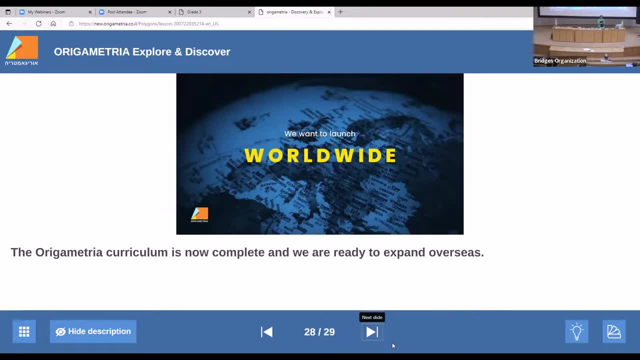 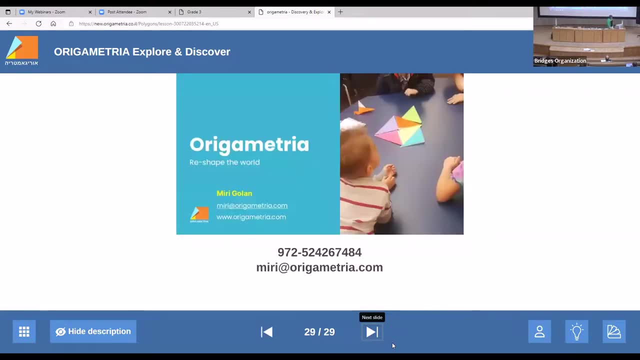 better result in geometry and geometry is better result in geometry and geometry is better result in geometry and geometry is important uh topics. so if any one of you want to have a contact with me, please do. and you got here the jackson cube so you can take it apart and build it if you want. this is how we give away to the. 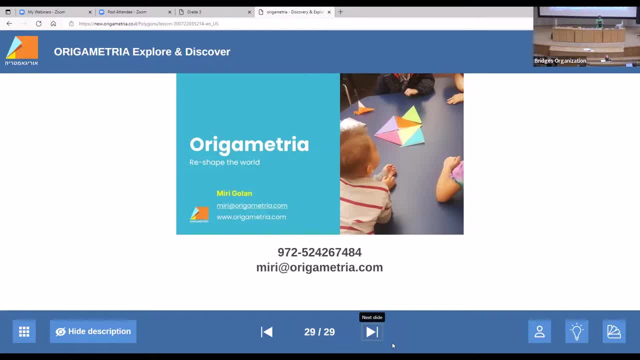 school to show them. yeah, it's origami, it's fun, but this origami teach you geometry, so i hope i open you some window to origametry and thank you. if you have a question, i'm here to answer. thank you for that great talk, um, so we'll start here with eve. 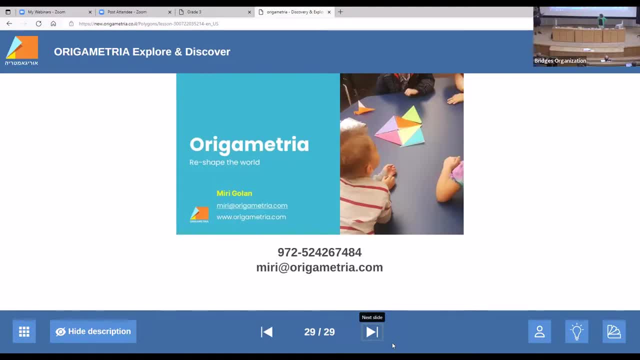 no, they need to pay. repeat the question. so the question was on the cost of the curriculum. um, i think, if anybody want to talk to me, but uh, yes, it's cost. you know, all this cost fortune to make the animation and hours of work. so, yes, usually school buy a membership for one year. 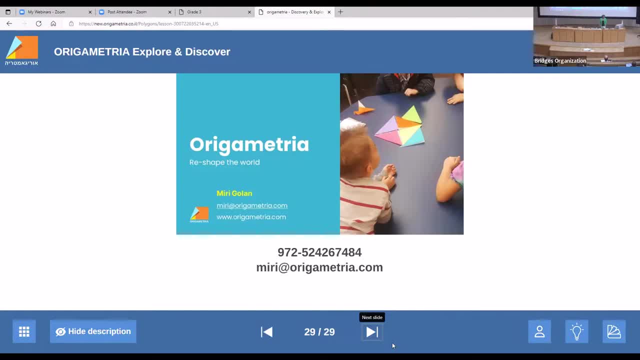 what can i talk to you later? but if somebody want price, talk to me about it later. it's not? yeah, so the question is about, uh, other topics beyond origami, other topics beyond strictly geometry. yeah, we start to make a salmon church session. um, with fraction, prepare the student for fraction, the problem with fraction that. 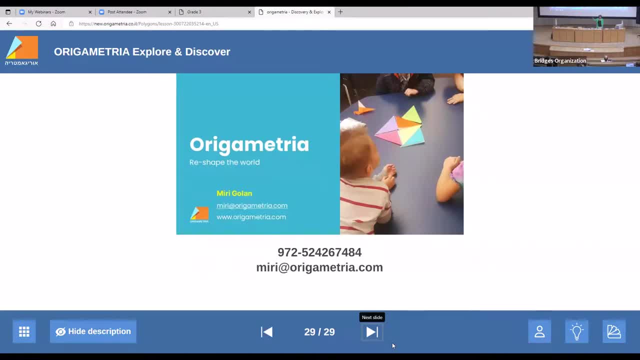 the teacher run to do quiz with the student before they understand what is a half, what is three, quarter, what is so what we did? we build a session. who build the geometry understanding of fraction? so they can do. we in the middle school we did go up and i think this year we're going to. 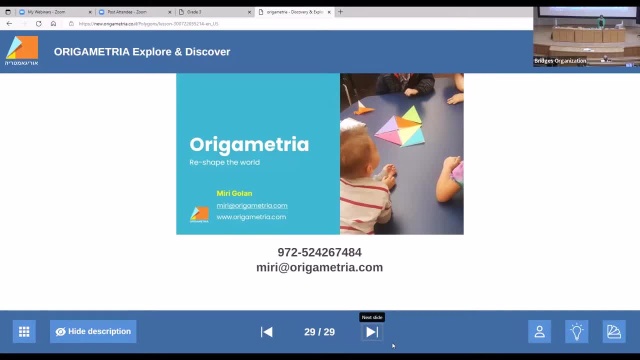 go and fill up more lesson to middle school and up. so i think every time we give more and more to um higher mathematics and also not just geometry touching the mathematics. paul, you have a question um. so the question is about: uh, how organized Orgometria helps children with learning disabilities? 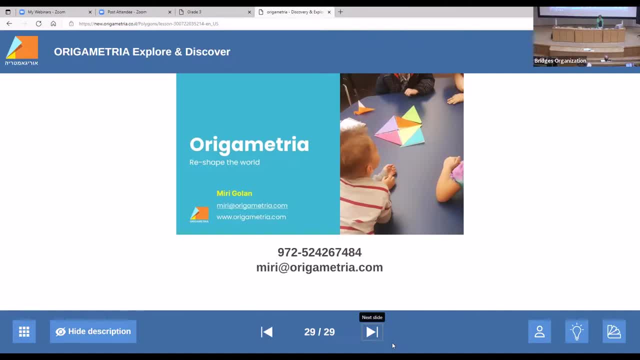 I start my way in the special education school. Children was there from intelligent average and up. but emotional problem and learning problem. Orgometria is very, very good for students who have dyslexic learning problem, hyperactive emotional problem. We have a phrase that I really like. 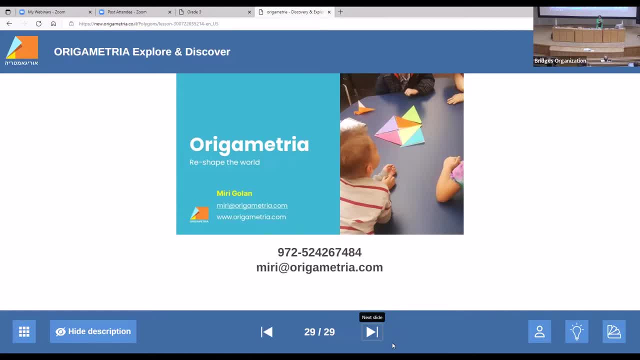 So when I start, I start origami also as a therapy. Yeah, And many of the students I teach now they are 30 years old And it's amazing what they tell me- this changed their life because they start the learning with Orgometria with me. 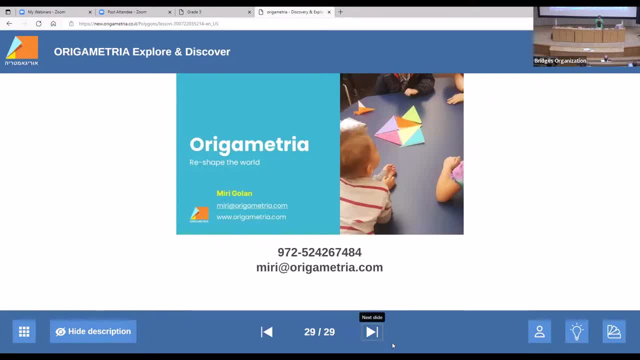 And then they saw they can succeed and go to the other area. So the phrase is: when the paper fold, the emotional unfold And it's everything you know. So in special education, yes, you can use it, And we all the time hear from the teacher. 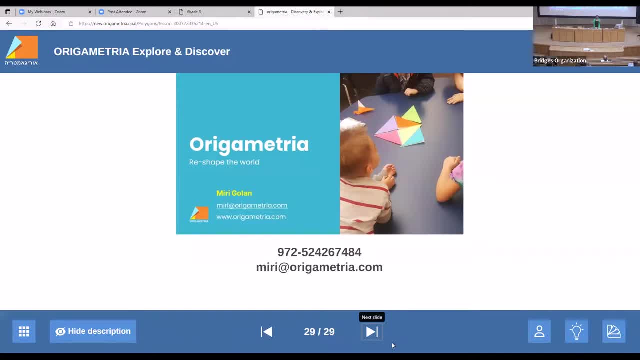 I always have kids in the class who doesn't work, He's not good, He's make a mess And when Orgometria start he sit the first and he have better result. So it is very good tools. Answer the question. 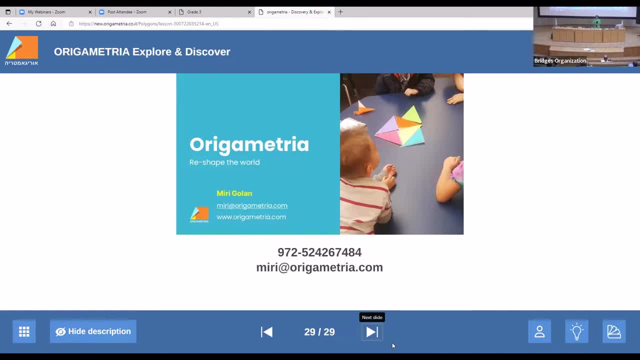 Way in the back up here. So the question is: are there learning theories that are used to frame the student thinking: Yes, I have a question. Yes, I have a question. Yes, we do teach, like Van Gila. you know when the children start to. when I train teacher, I talk about Van Gila a lot because I think it's very important. 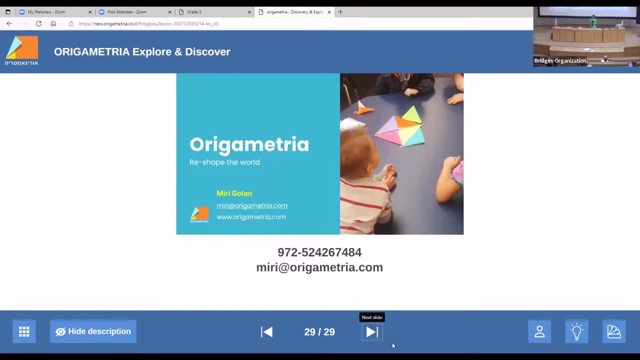 They did it in 1950, but it's still relevant, Yeah, So sometimes the teacher escape. Don't teach In kindergarten, don't teach first and second grade. Start third grade. Now they need to understand angle, but they don't know what is a polygon. 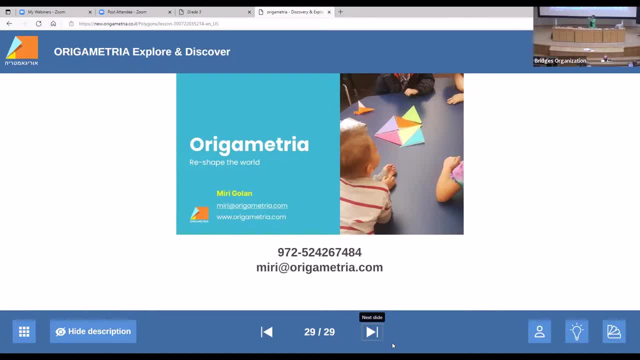 They don't know what's the size. They don't know. So a lot of material is missing And while the teacher teach and the children doesn't understand, it's not because the children have no ability, It's something missing. I always say to teacher when I train them: 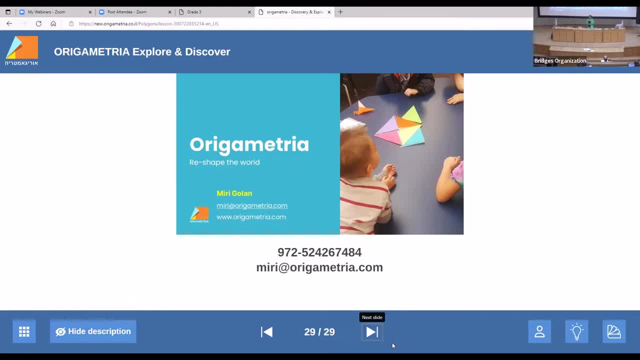 When you try to teach something And the student don't understand, don't continue to try to explain in the same from a different direction. check what he miss, what's missing of his understanding. Now I asked the the if you, if you understand what's missing and you teach him what the missing material, he'd be okay. 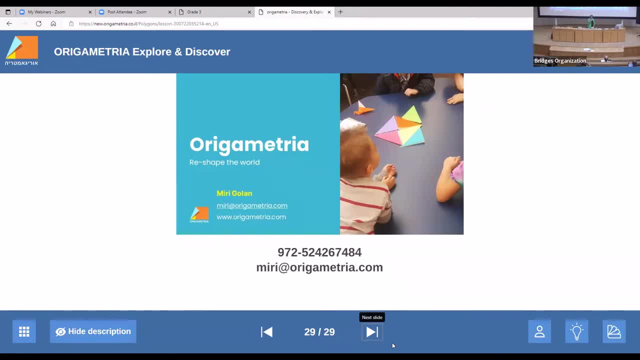 And I asked my teacher what's the most important thing happened in your class? There's so many thing except one. it's the student answer. If he answer me and I listen to his answer, I know what he doesn't know. I know what he know. 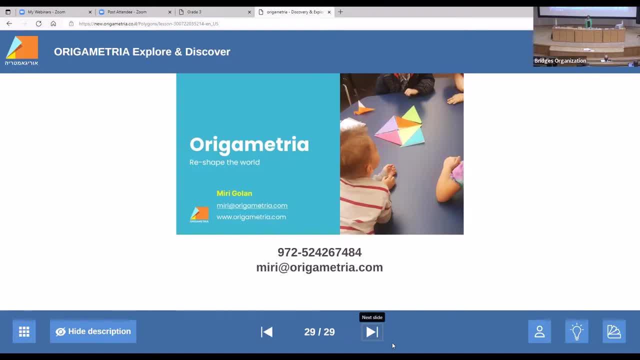 The answer is very important. You know the education system run too much to exam. They say exam 60,, 90, hundred. What's it mean? What it say about me If I have 90 or 60. ah, they said i'm very good or very low, and this is wrong. i think the exam in the beginning starts. 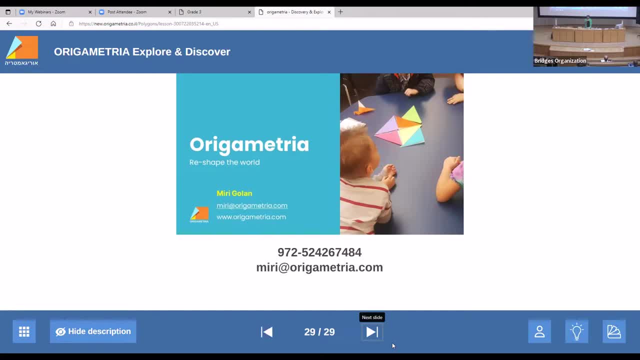 to let the teacher to understand what the student missed so they can complete and be okay, and instead we turn that is, the student is good or not good, and this is wrong. that's why when my son came up to me within 160- 40, i never say to him very good, i always ask him: are you happy with? 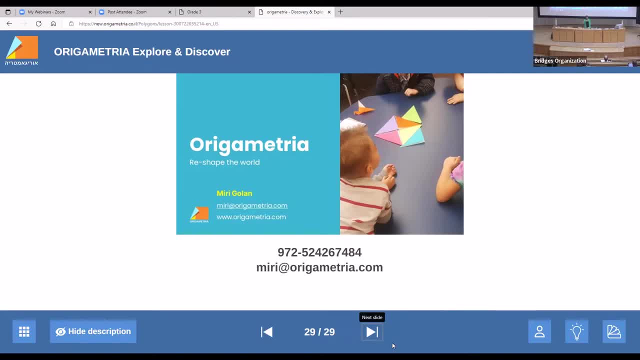 that this is what you want, is it okay for you? and sometime he got 70 and he said i'm very happy and i need to say okay, it's very important not to so all what you talk about um vanilla and teaching um according to ability of the student. it's very, very important to understand that, because i see many 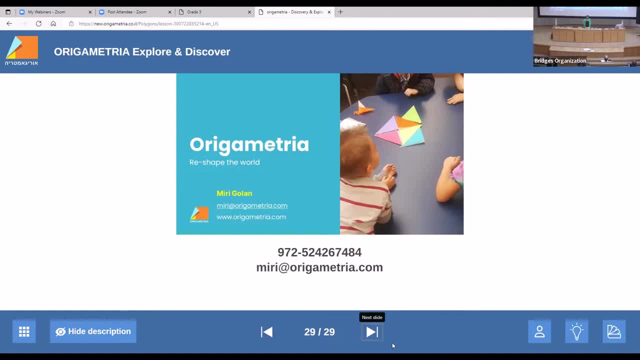 teacher who doesn't understand it. they try to explain that the student doesn't stand, say oh, he's not good in math. it's not true. everybody can be good in math, everybody can be good in geometry. just teach, right. yeah, the question is: um, is this, uh, this teaching methodology, uh helpful in students constructing? 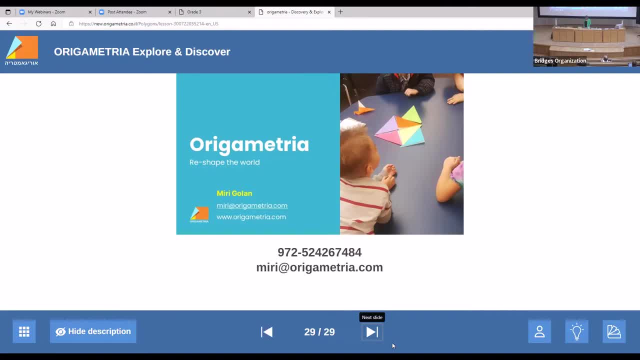 proofs later on in a more formal way help people. i just said the question. so are the when students are doing this, um, do you have evidence that perhaps later on in school that they do really well in terms of being able to formally prove things in a written way, in a? 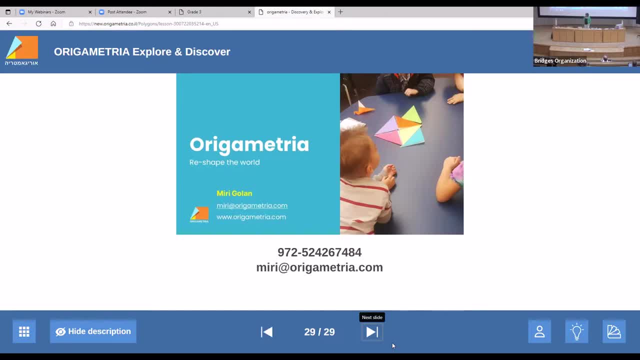 geometry class or subsequent courses that they take, the thing is, before they did the research, i knew it. i hear that. i heard it from the teacher, because if the teacher died for the four years it's mean you're doing something. so we hear that all the time. i'm i'm working with that, for you know, teaching with origami for more. 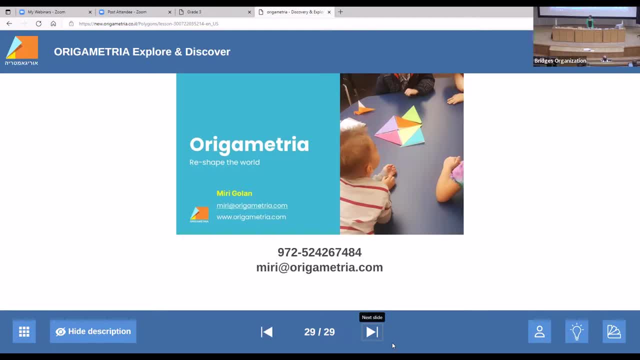 than 30 years. i see all the time that i hear my students when i was young and i was teaching them. so, yes, we know it, but it's not enough that i tell you that i improve and they come to me. the most important will be more and more research about it, when people believe it better. yeah, but yes, 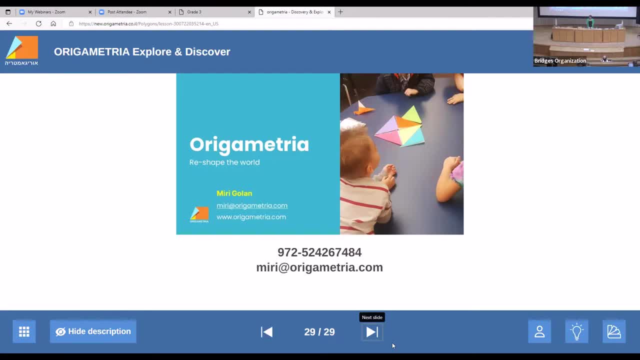 if you use it and you know it. you know what i said to a principal, because sometimes teachers have they say i don't want to teach it, i don't know if i succeed with origami and all this. so i said to the principal who buy the program: tell your teacher that you're going to come in. 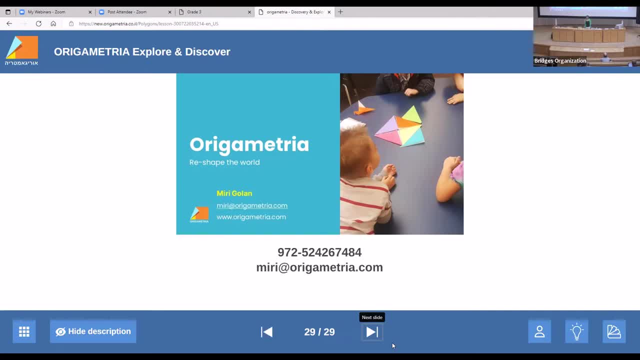 the lesson they teach, origami tria. so they should teach and you come. you don't have to come, it's enough. you tell them you come or maybe come for five minutes. so if the teacher know the principal, come to watch her. she start to practice and start to teach what's happened when she start to teach. 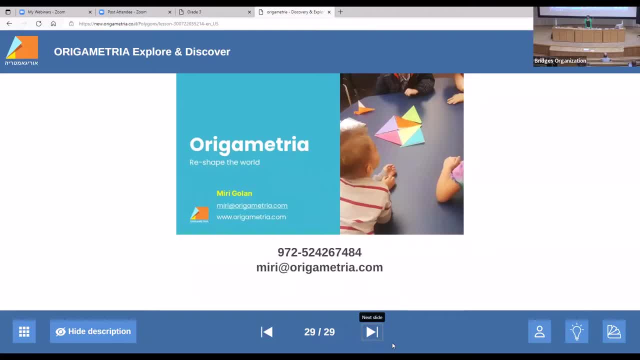 the children get crazy about it. they don't think they enjoy the investigation of the geometry. they have some origami model. they love it and then start to knock the teacher: can we study origami? can we study origami? so it's came from the children and put pressure to the teacher to. 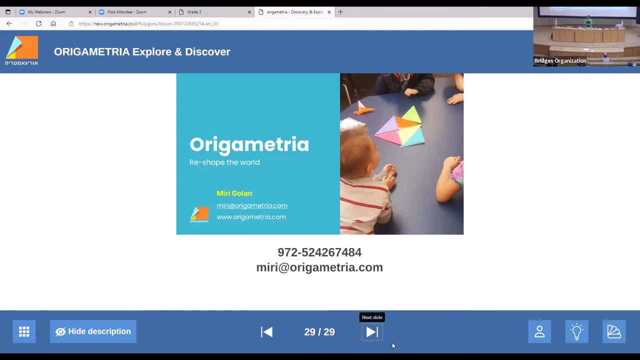 change to to take something she doesn't know that this can improve, and after she give them exam and she or the math supervisor in school suddenly see the result is up, of course they take it. he said any more questions, so so the question is: um, what is the debugging process for the pedagogy that is involved in uh? 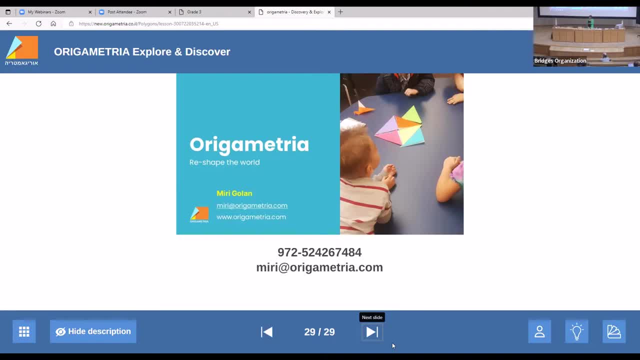 this organization. You give example that the students fall wrong on what you do. You know that's what you mean. Okay, After every step we teach, I recommend the teacher to go between the student. We never say to them: it's beautiful, it's good. 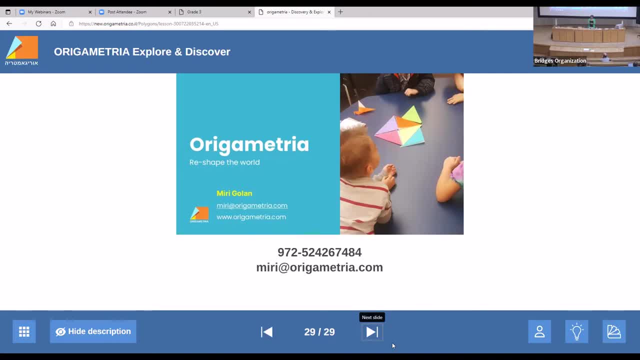 We say to them: ichiban. in Japanese Ichi is one, ban is thousand. You are champion. Now, ichiban is a word nobody use, Only the origameter teacher. She go between them and in every step almost. 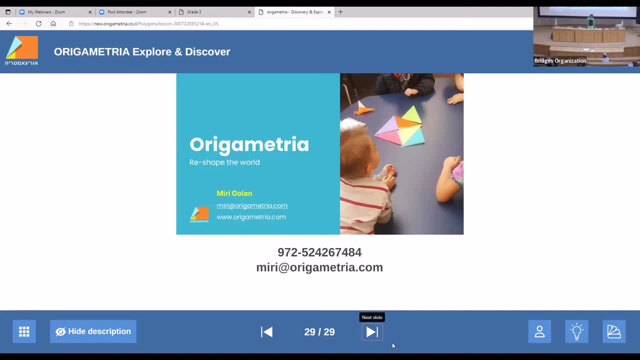 And see she always go in a random way. She doesn't go straight to the kids. who doesn't succeed, Because he feel like she help me, she didn't help anybody. Then it's become worse. So she make kind of a right, all the time going in the same direction. 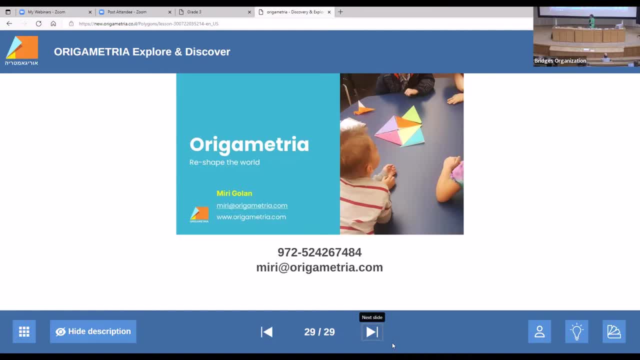 And she give ichiban to everybody. So if I give ichiban ichiban and then he have a problem, If I stop a minute and show him with my paper, Nobody feel and he feel more confident. So it doesn't happen that after few step that you find out that he didn't fold it right. 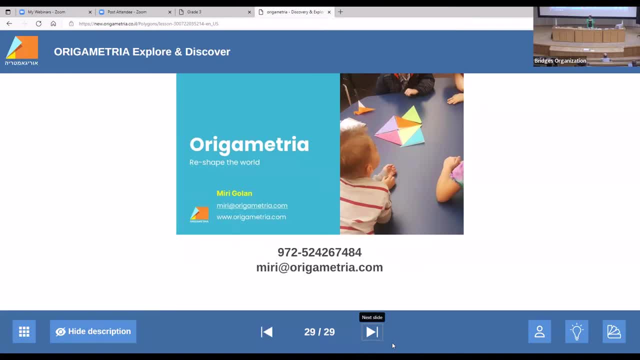 We don't come to this position because we all the time see the student and go over. I hate the word succeed. Very good, you succeed. I hate this word Because when I work in a special education, I ask the student why he didn't succeed. 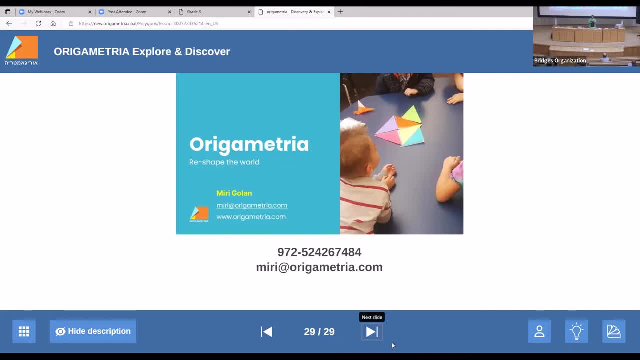 The answer I got: I'm not good enough, I have no ability, I'm not good. So when you say succeed, or even you praise as you did successful way, you know I hate this word because the students stop to try, because what is learning? to try again and again. 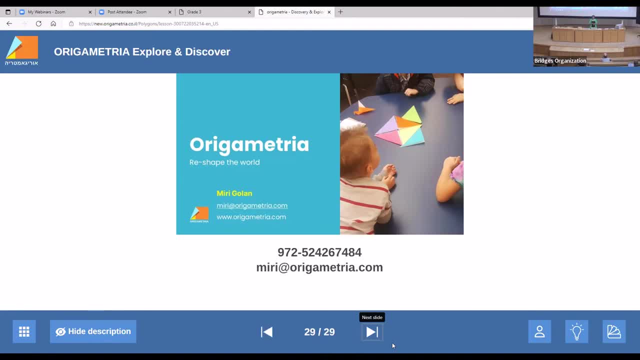 And there is a word that I say it's adult world. We learn from mistake. Doesn't work for the student What we learn from mistake. If I say I did bad, I'm not good, And they stop trying. So I tell my teacher: open the window, throw the word. 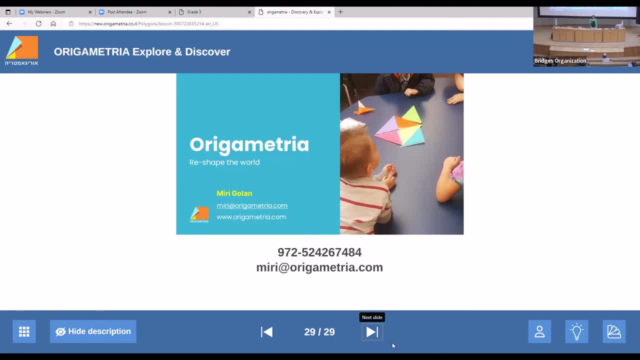 Succeed out of the class and say: did you find it is discovered that in Hebrew we say it's a nice word. Did you discover that? Did you find it? Why? So ask the student why you didn't find it. 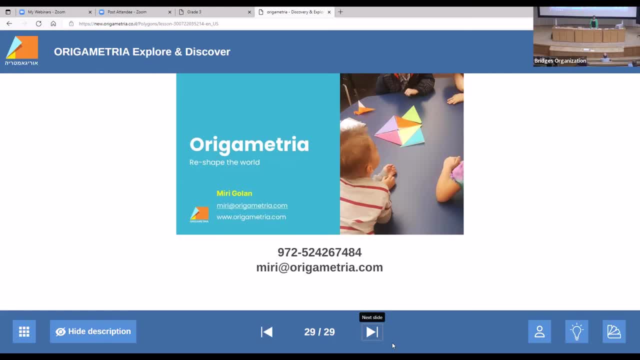 I don't know. I find it later. Why didn't discover? I will try to discover after. it's not me The word success, It's my ability And I don't like it. So we take this word out of the class. 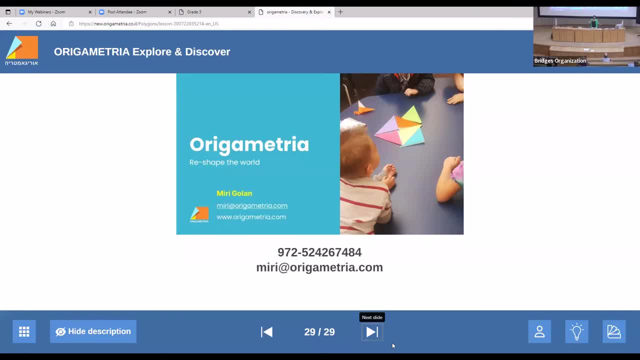 I sometime I give you know, I teach the teacher to teach origami, but many times I give the method. The principal come to me and say you know all the years to talk about it. because of what? 20 years in a special education. 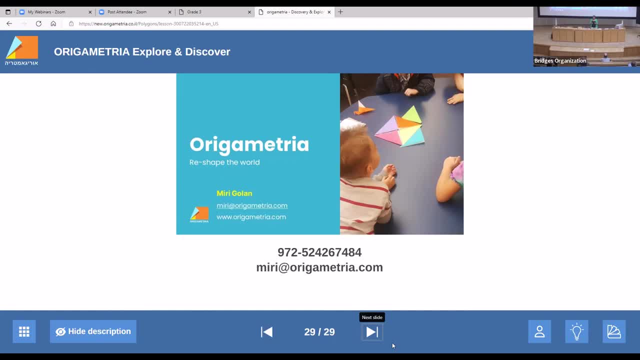 I have big understanding. What's wrong? What stop the student to try? We need the student to try all the time, because learning is to discover, is to find. it's excitement, It's curiosity, It's not to know a knowledge You open Google. 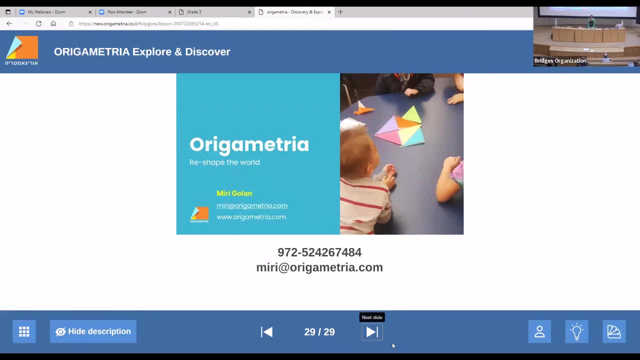 You have knowledge in two seconds, Something important. but to make them, If I finish my lesson and the students still try to find out or open out the holes, try to find more trapezium, I succeed If the student take it, put it in the bag, the forget about it. 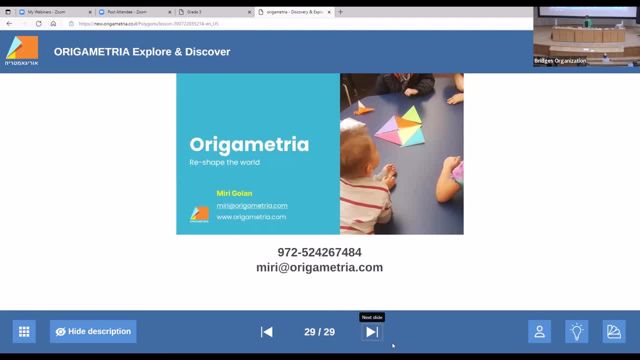 I didn't know what they did. So at this point it is 1030,, which means that it's time for our coffee break. Yeah, So what that means is that everyone can go get some coffee, stretch your legs, but come back here at 11 for our next speaker.